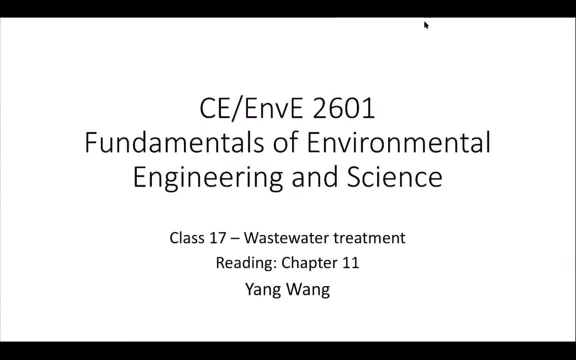 Okay, yeah, so it's already 11 and I think we should get started. So from this class on, we're going to learn about the wastewater treatment. Okay, so we spent quite a lot of time talking about the chemistry, talking about the basic chemical concepts, And then, in the 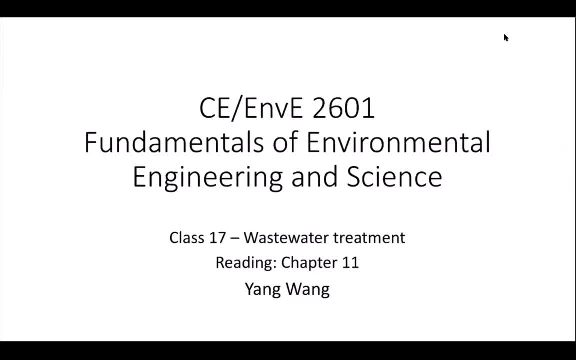 second quarter we may introduce the water treatment, which is mainly for the drinking water. Okay, so now we're going to jump into the wastewater treatment, And actually a lot of the processing or a lot of the treatment methods are quite similar. 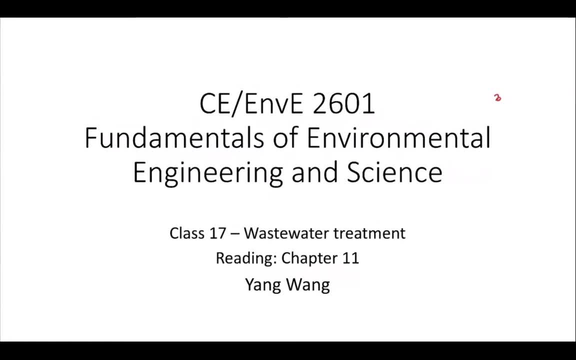 And the wave. yes, I said a lot of contents are going to be quite similar, So I think we're going to have a smooth, smooth third quarter here, Right, So I also went over the exam that you already submitted. I think most of 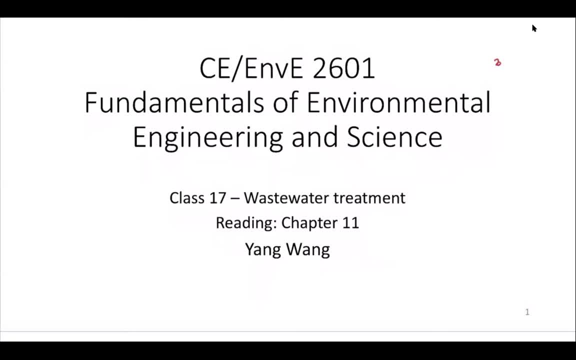 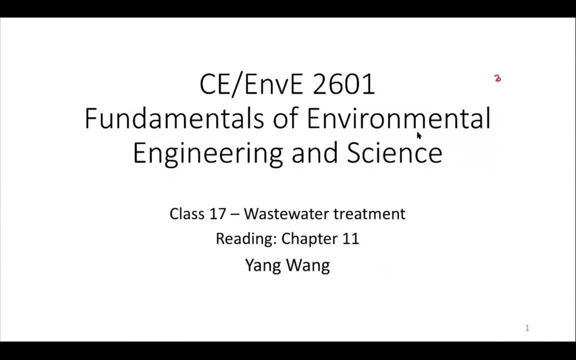 you guys did pretty good, As you can see. for the exam problems, they're mainly focused on the design parameters, right? It's quite straightforward And we have the conditions and we can calculate what are the design parameters for the system, right? So hopefully I can get it graded. 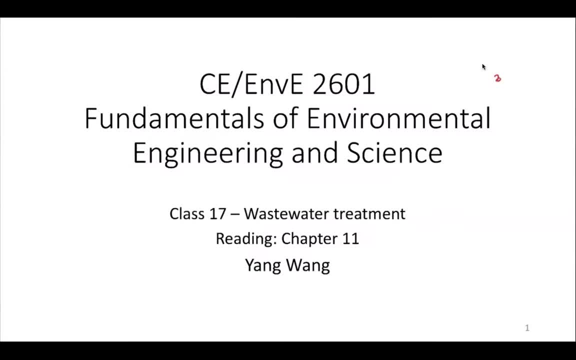 Let's say, before the end of next week. okay, so well, during this time, if you have any questions or if you feel that you didn't perform well in the exam, feel free to send me an email. we can discuss what is going on and come up with some solutions. Okay so, 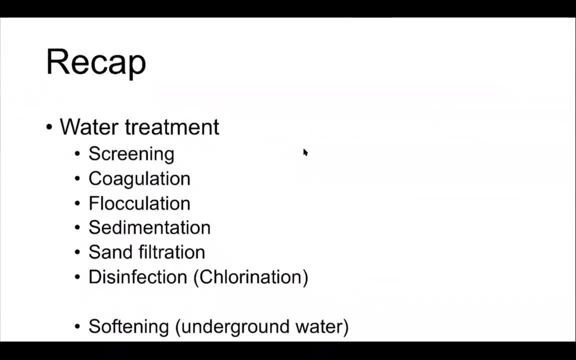 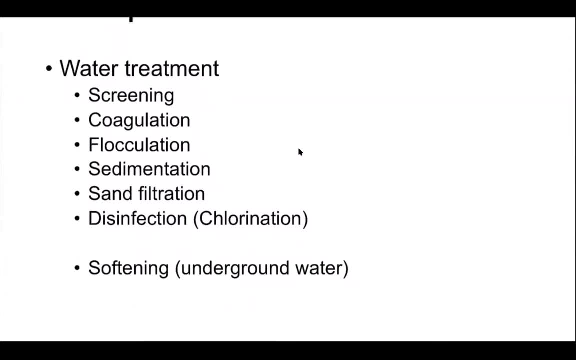 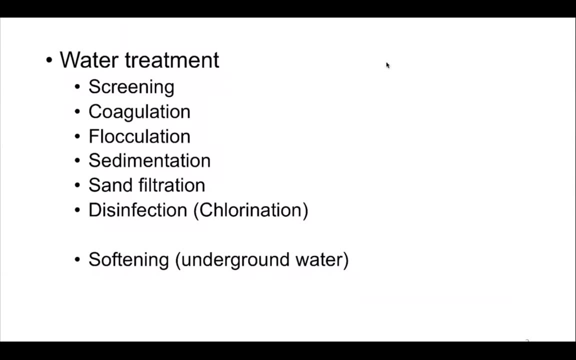 so let's again do a quick recap of the basically last chapter. So last chapter we talked about the water treatment. Specifically, we said water treatment is equal to drinking water treatment right And because it is directly delivering to the human for people to drink. So the water treatment is going to have a much more stringent standard right, and the processing or the treatment methods actually more. 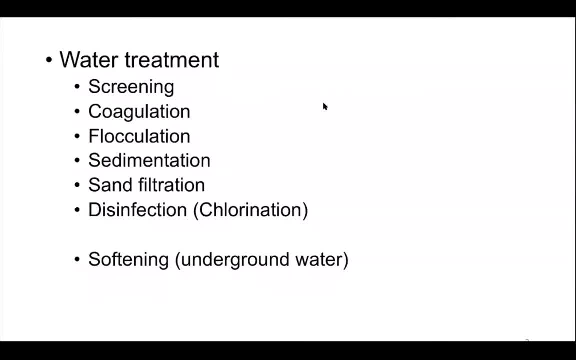 complex. So what is happening is that for the surface water, let's say for the lake or river water, It's composed of of these processes, which include the screening, the coagulation, flocculation, sedimentation And then, basically, after all, the larger particles. 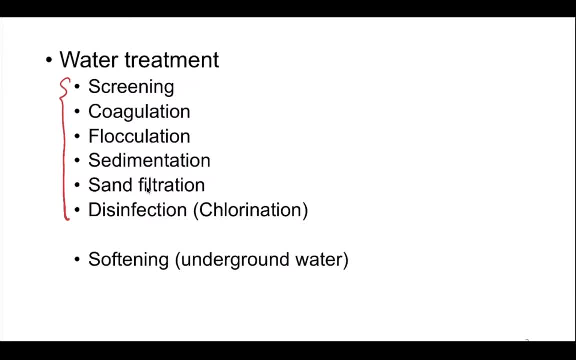 are settled down, we send the water through a scent filtration to remove the smaller particles And finally we have the disinfection to remove the living organisms, let's say the viruses or bacteria, before we send it out to the host tools, right? 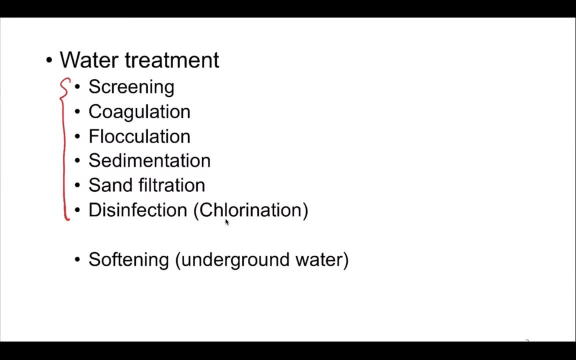 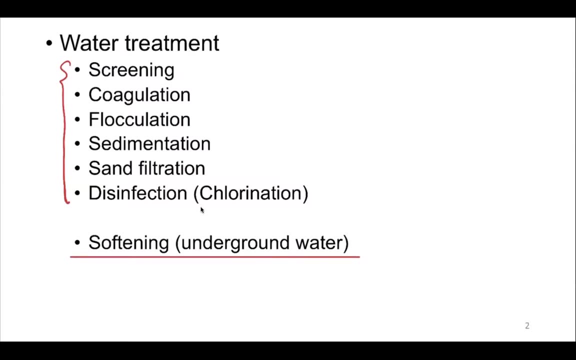 So that process is also called chlorination, because this is the most common chemical that people use to kill the pathogens right? So we also mentioned that for the groundwater the softening is going to be more important because there are a lot of hardness ions. 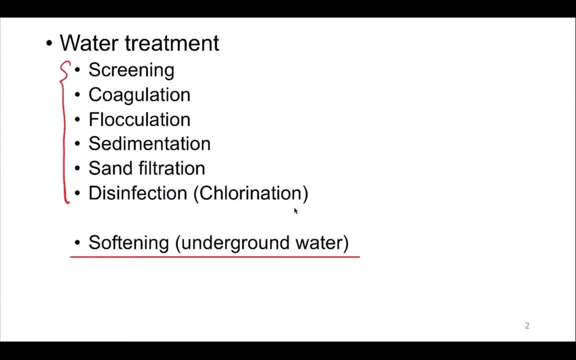 let's say calcium ion, magnesium ion, and we want to basically reduce the hardness or soften the water So that they don't settle down onto the pipes right Or people don't ingest too much of them. So these are the general methods for the water treatment. 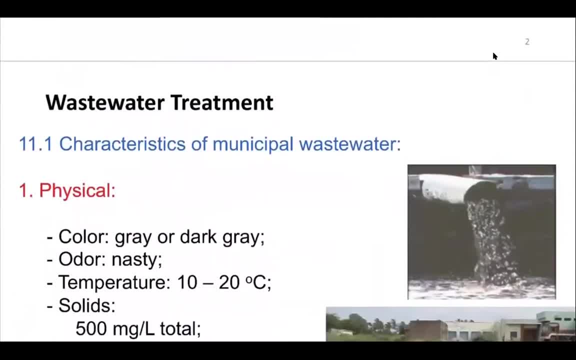 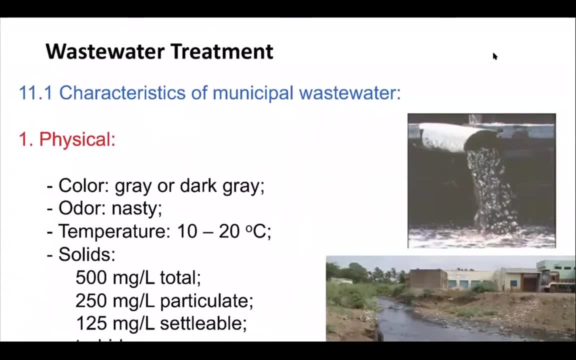 And in terms of wastewater treatment, as I said, a lot of the processes are quite similar, except that we're dealing with a much more polluted water. If you compare, let's say, the water from the lake or from the river, they're going to be much more cleaner. 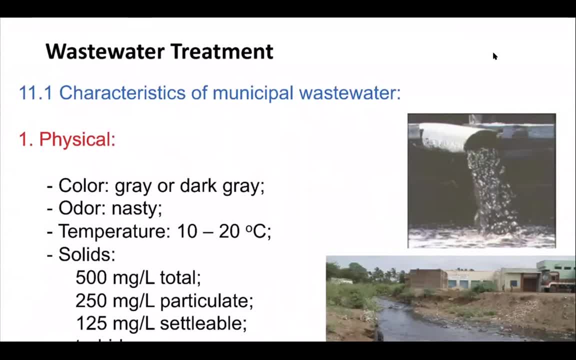 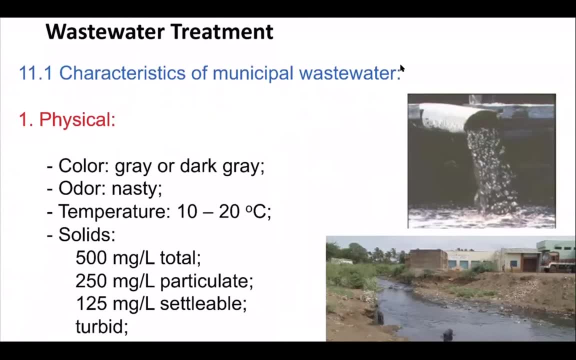 and they have less contaminants in there. So because of that, we need to first know what is the characteristics of the wastewater. So here, what it's showing is the properties of the municipal wastewater right. So these properties are going to include both the physical properties and chemical properties. 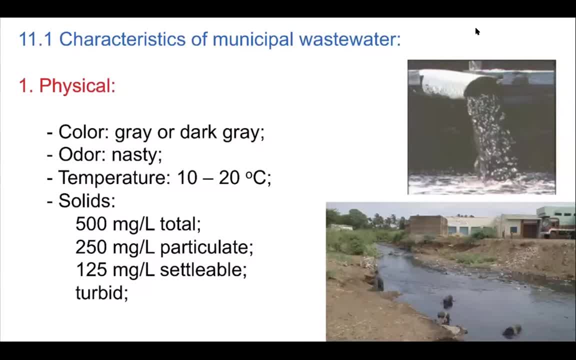 So first, on the physical, what we know is that the water for the wastewater generally looks pretty gray or dark gray, right, It doesn't matter, It definitely doesn't look clear, right. In terms of the odor, a lot of them are very nasty, right? 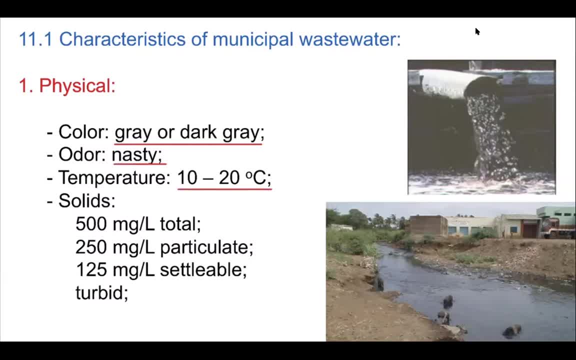 In terms of temperature, it's around 10 to 20 Celsius And this is mainly because, in terms of the wastewater, either coming from the residential area or the households, or from the industry, people normally operate it under normal temperature. It's under very rare situation that people will use. 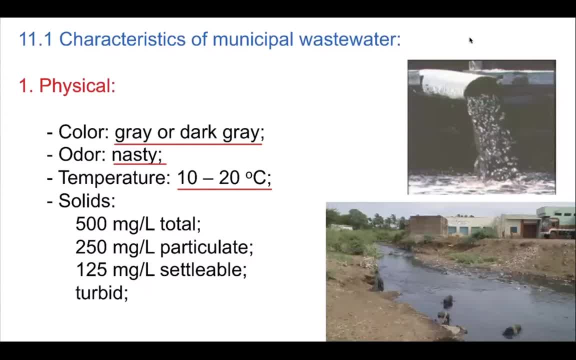 or generate wastewater under the freezing point right, So the water is filled with a lot of solids inside. So in terms of these suspended solids- what people call suspended solids- so the total amount is around 500 milligram per liter. So it's around 0.5 gram per liter, right. 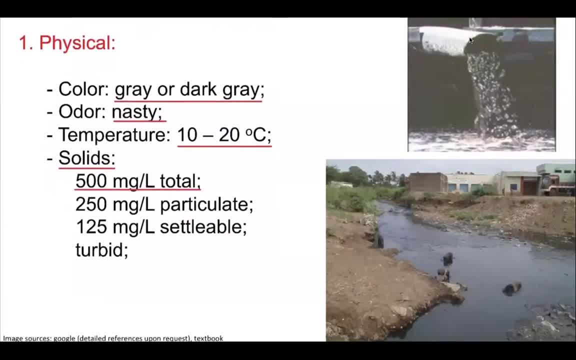 And half of them are particulate, okay, So they can suspend in the water for a very long time. It's like the colloids that we described right. It's like the colloids that we described right. It's like the colloids that we described right. 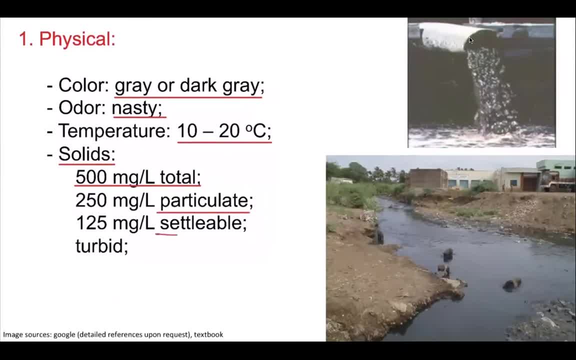 And then further a quarter of them are settlable, which means that they have a larger size And if you give them enough of long time, they can settle down onto the base, settle down onto the bottom And, because the wastewater has a lot of solids, 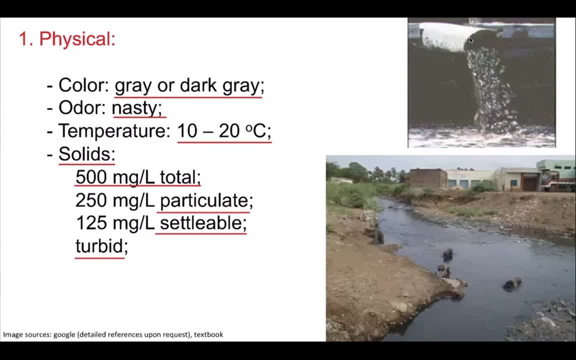 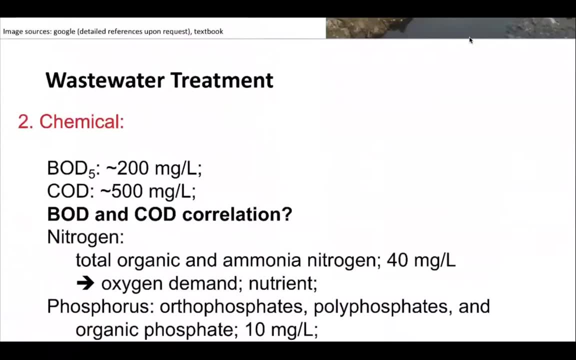 basically, the water is going to look very turbid right, And that's why we have to deal with these contaminants or pollutants. So this is the physical property And, in terms of the liquid, we have a water that has a lot of solids. 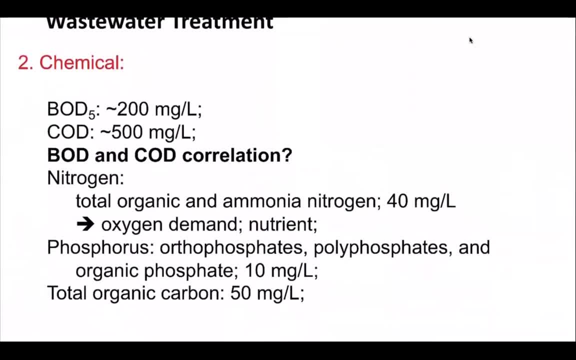 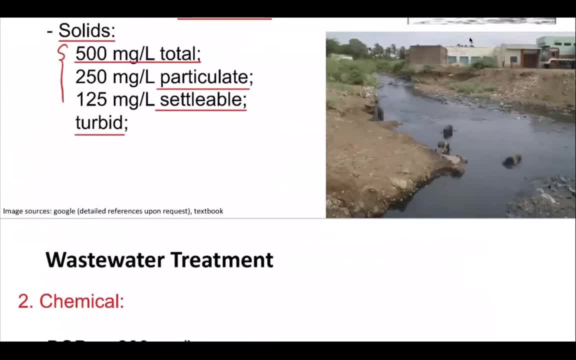 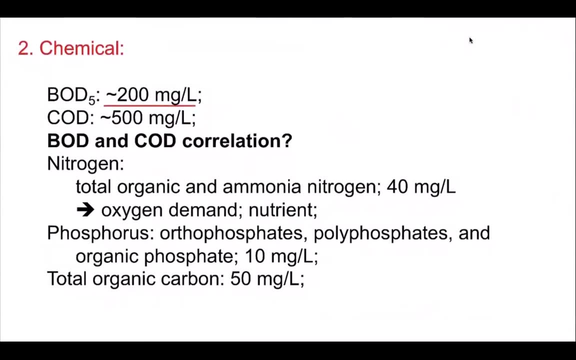 of the chemical property. So here what I'm showing these numbers and including numbers shown in here. these are just some general numbers, Let's give you some understanding. let's say the approximate value or ballpark of the contaminant level, but the detailed wastewater property, really. 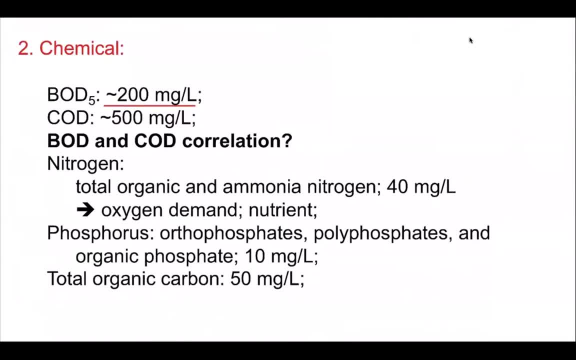 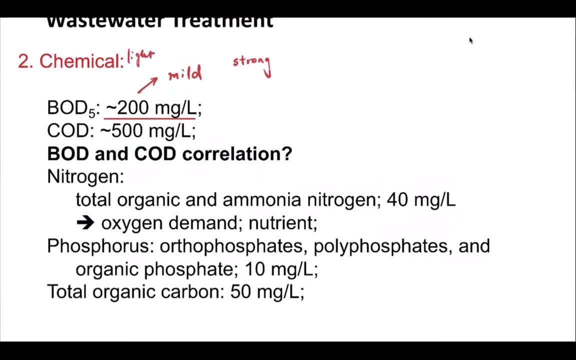 depends on the source. So if you further look at the table in the textbook, actually these numbers correspond to the mild condition of the wastewater. So people can also have strong or strongly polluted wastewater or lightly polluted wastewater. So this is just a mild condition which is for a lot of time, the general condition. 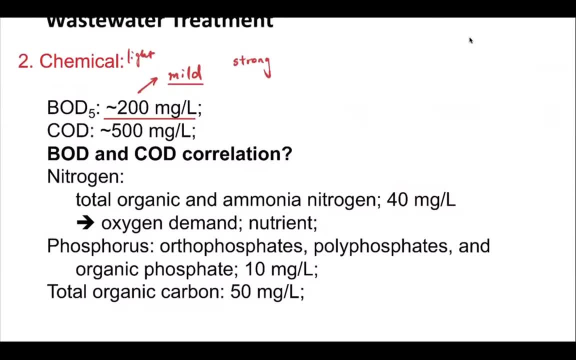 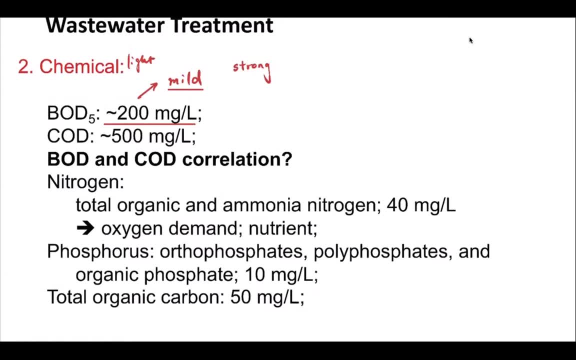 So in terms of the BOD5 for the wastewater, it's around 200 milligram per liter. okay, so we mentioned that the maximum dissolved oxygen is around 8 to 8.5, right, So what this means is that the BOD is. 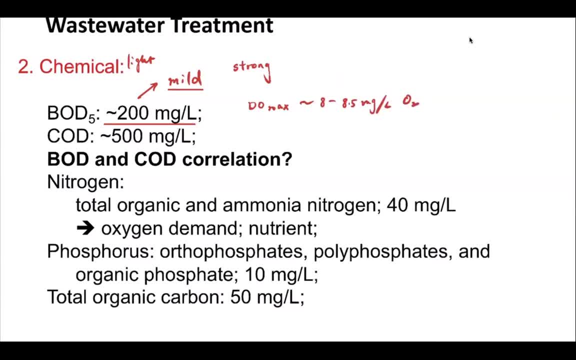 too large. So actually you can calculate what is the oxygen content of the BOD5 and the BOD6.. The BOD6 is the ultimate BOD. BOD0, right? So the ultimate BOD is definitely going to be larger than. 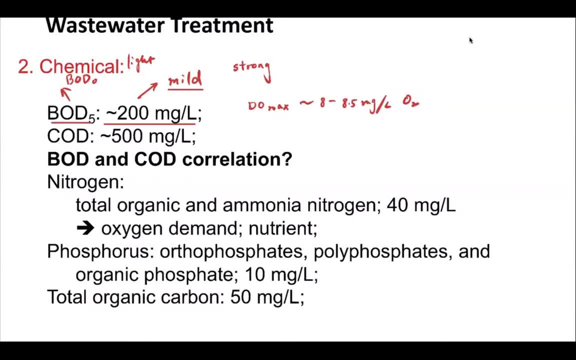 the BOD5.. I think we also had the exam problem in the second exam, right? So you can calculate that based on the rate constants. So what this means is that there's no way any living organism can live in this wastewater because, simply because you don't have enough of oxygen, right? All of the 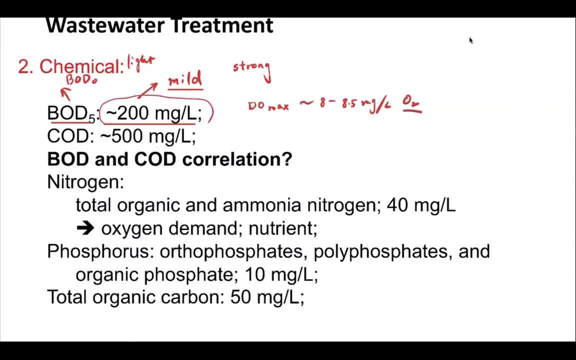 oxygen are consumed and you have so large amount of BOD5. So the BOD6 is going to be larger than the BOD5. So the BOD6 is going to be larger than the BOD6. So the BOD6 is going to be larger than the BOD5.. 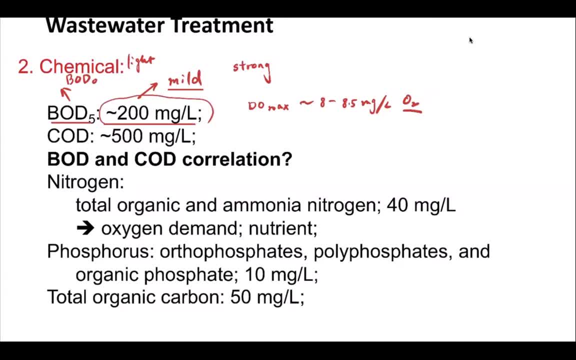 So the BOD6 is going to be larger than the BOD6.. So the BOD6 is going to be larger than the BOD5.. So people also measure the chemical oxygen demand right. So the chemical oxygen demand is around 500 milligram per liter. okay, So just as a recall of the oxygen demand here. So here I have a first. 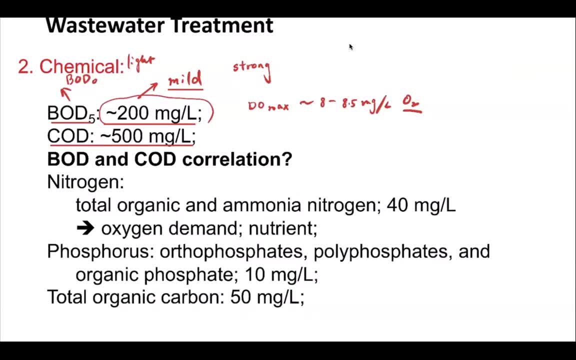 quiz problem which is asking for what is the relationship between the chemical oxygen demand and the biochemical oxygen demand. Okay, so we'll give it five more seconds for you to choose the answer. Okay, so I would say almost all of you got the correct answer. Okay, so the COD is always. 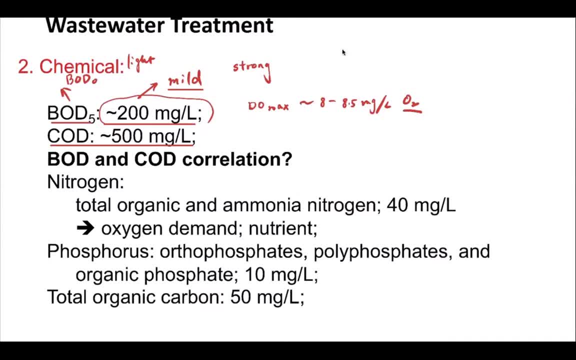 larger or equal to BOD, And this is not because of the number that I show here. Okay, so the COD is the BOD. To compare these two, we need to first convert the BOD5 into the ultimate BOD right. We know that the ultimate BOD is larger than 200. 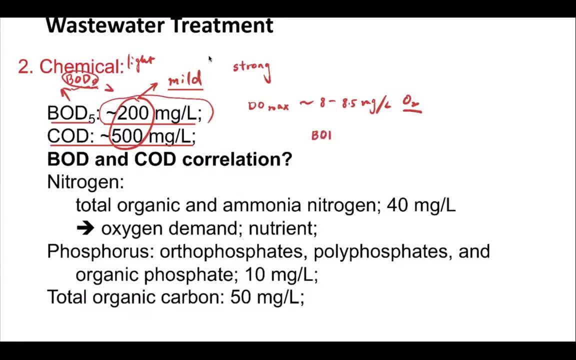 But in terms of the ultimate, even if we compare the ultimate BOD or the ultimate COD. okay, So what we know is that the COD is always larger than BOD. This is mainly because the biochemical oxygen demand only talks about the organics that can get consumed by the bacteria, right, For example, the plastic bag or plastic. 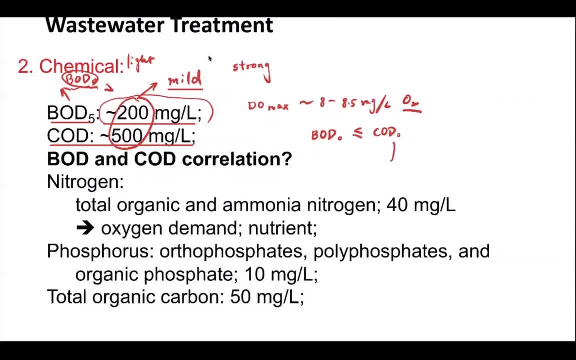 bottle. They're considered in the COD because they are organic, right, They're organic. but the bacteria or the living organisms, they cannot consume the plastic materials right. So that's why the BOD is normal. We have to do something else. We have to have an economy. right, We have to용 within thather and that would be a Η framework. And so that's what the COD like, the sustainablestein vaporization means that they cannot consume the plastic materials, right. So that's why the BOD is normal COD, the chemical oxygen demand. Okay, so you said it. 2 sex hug suit is a farm sure thing to talk to. but 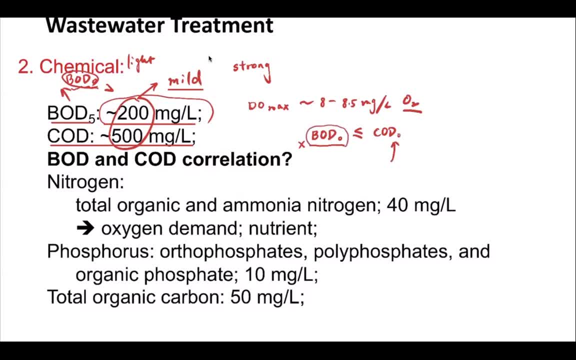 normally smaller than COD, or it has to be smaller than COD, And at the same time actually a lot of the organics. when they're being consumed by the bacteria, they became a part of the bacteria, right? So not all of them are converted into carbon dioxide and water, So 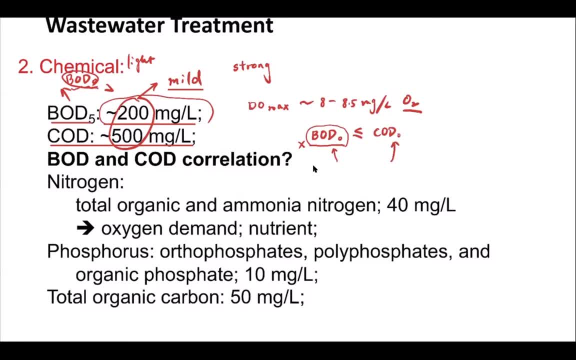 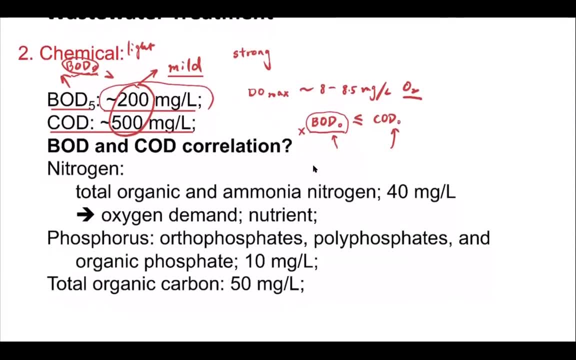 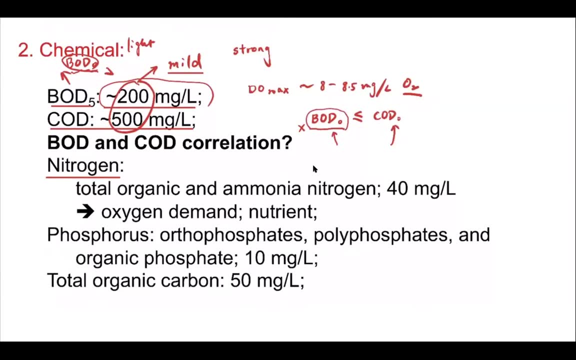 that's why COD is always equal or larger than BOD, okay, So I'm glad that you still can recall this concept, right? So, in terms of the chemical properties, we also discussed the nitrogen, right? So the nitrogen in the wastewater is also under a pretty high concentration, So it can. 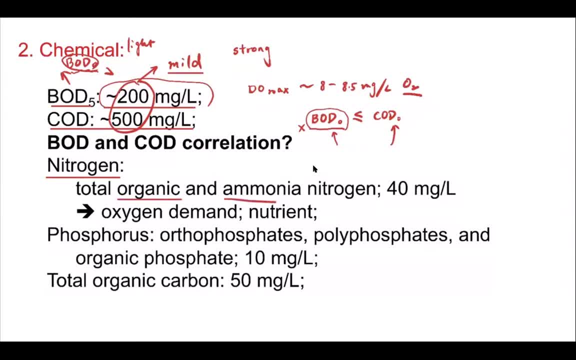 include both the organic nitrogen and ammonia nitrogen- okay. So basically you can include some organics, let's say carbon, attached with nitrogen, right? You can also have the nitrate ions- okay, And ammonia Ammonia ions, right. So their concentration is around 40 milligram per liter, So the nitrogen is. 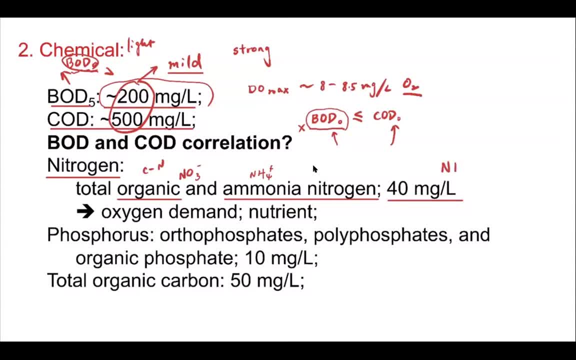 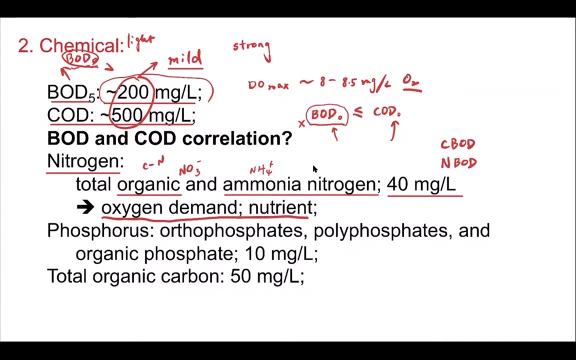 quite important also because we discussed the concept of NBOD, right, The nitrogenous BOD. So there are CBOD, the carbonaceous BOD and the nitrogenous BOD right. So they're going to cause the oxygen demand And actually they're also a type of nutrient that's causing the 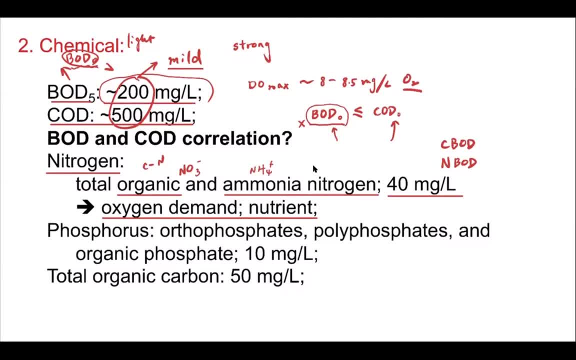 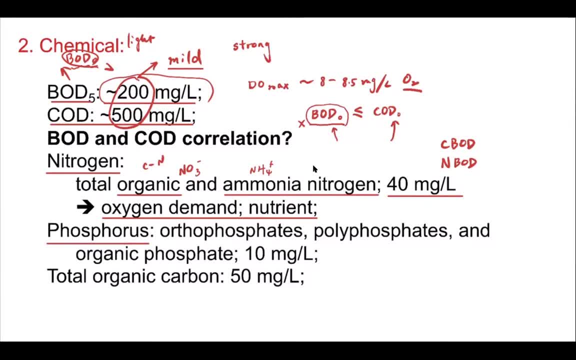 learned about is phosphorus. Phosphorus can exist in many formats, or the many chemicals, For example the orthophosphates, polyphosphates and organic phosphate. So their concentration is under, let's say, tens of milligram per liter. So there's also total organic carbon. It's the 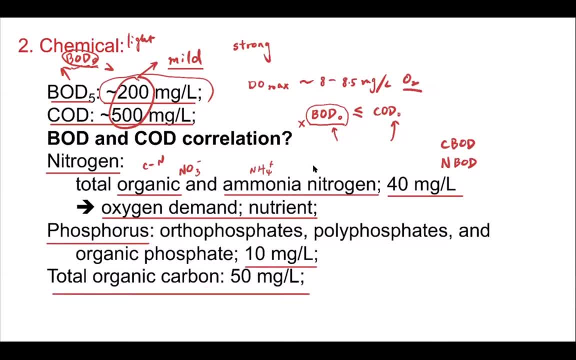 around 50 milligram per liter right. So generally the contaminant concentrations are much higher compared to the surface water And that's why it's also called the wastewater right, Because the contaminant concentration if it's lower than the surface water, we can directly discharge them. 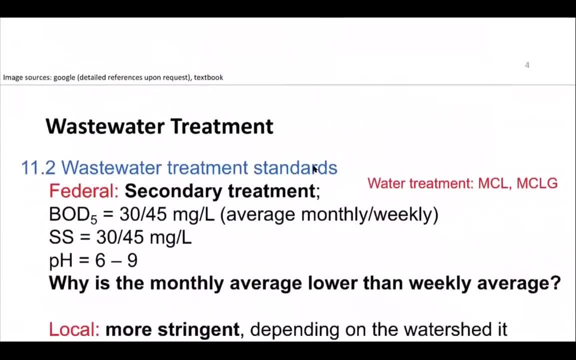 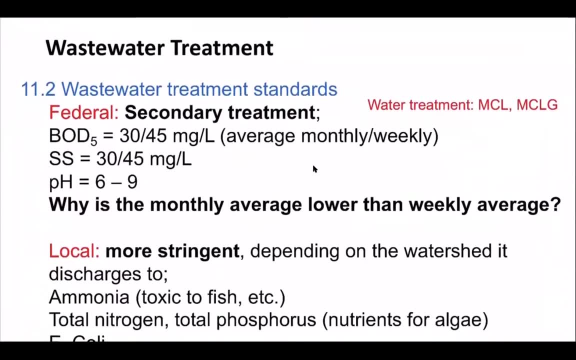 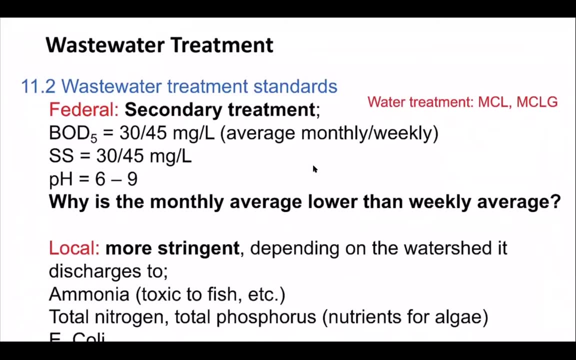 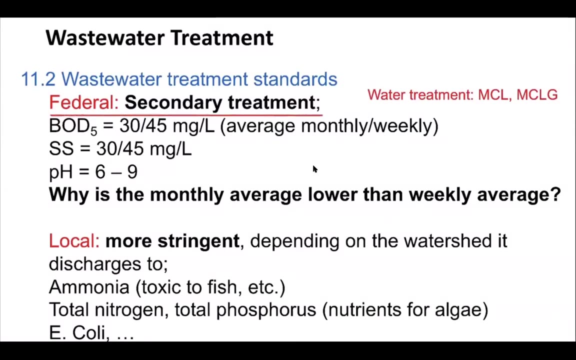 without any problem. So because it's contaminated. so the federal agencies, they set up standards for the wastewater, So we have to treat them before we discharge them into the surface water or underground. okay, So in terms of the federal requirement, they basically this is a normally. 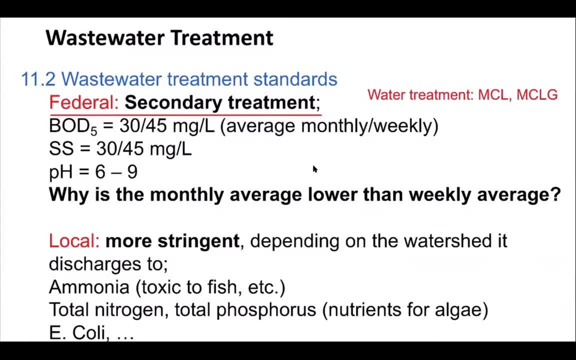 this is a more. it's a less stringent requirement, but it still requires a secondary treatment. So we're going to learn later on what this means. So, basically, for the wastewater treatment you have, you can have the primary treatment, but you can't have the secondary treatment. 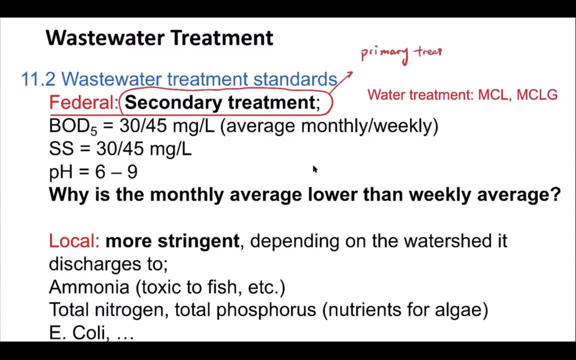 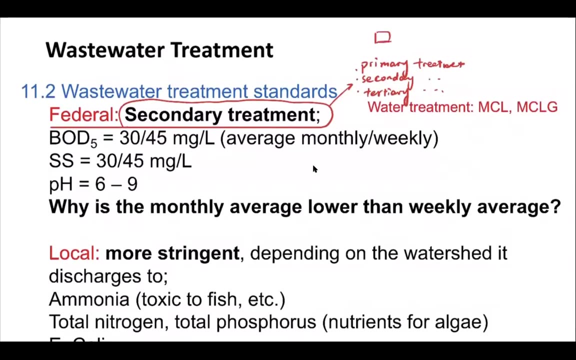 Okay, you can have the secondary or tertiary, Okay. So basically these treatments are going to get conducted in tandem, in series. So basically the first step is the primary treatment and then you can have the secondary treatment, tertiary treatment, and then you can discharge it. 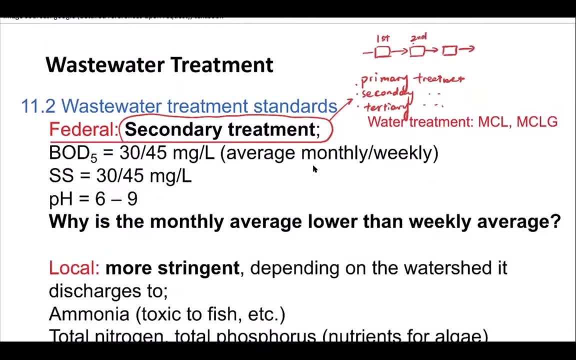 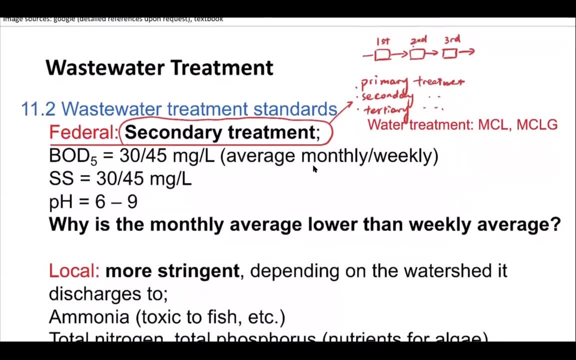 Right. So if the so, if the water quality for the wastewater, let's say in the industry or household, it's pretty good. So we can just use the primary treatment. But in terms of the federal requirement, what the what the requirement says is that you have to do a secondary treatment before. 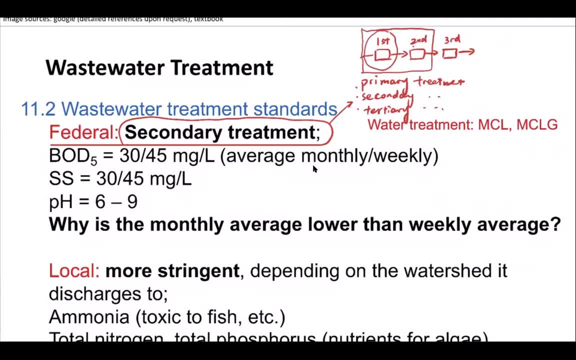 you discharge it into the surface water. Okay, So basically the first, the primary treatment, is a more simple method. You can just use the sedimentation to remove the contaminants. But the secondary treatment normally involves some biological processes, So we're going to learn more about these processes later on. All right, 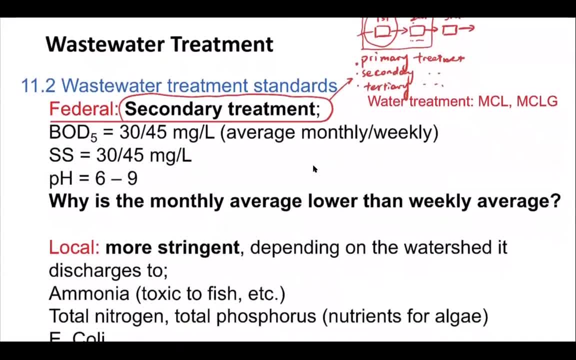 So this is a requirement in terms of how complex the treatment has to be. So they also give out a requirement for the treatment to be as complex as possible. So they also give out a requirement to be as complex as possible. So they also give out a requirement in terms of the concentration. So for 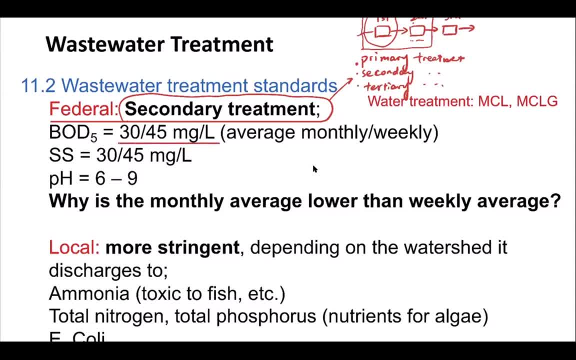 example, the BOD-5 has to be 30 in terms of the monthly average, or 45 milligram per liter in terms of the weekly average. So basically, what this tells is: let's say, a wastewater treatment plant, WWTP, wastewater treatment plant- discharge water out of the facility. Okay, So they will conduct. 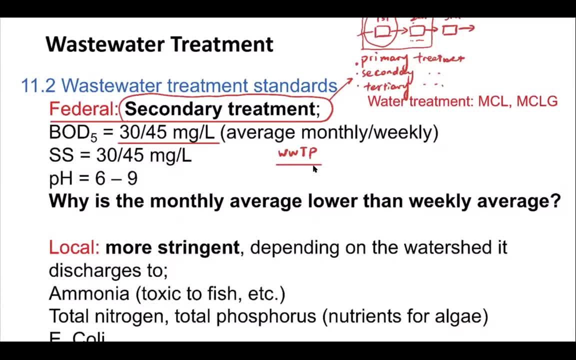 weekly or monthly measurements to make sure that the BOD5 is below 30 in terms of the monthly average or 45 in terms of the weekly in terms of the weekly average. So now we may have a question. So why the monthly average is smaller than the weekly? 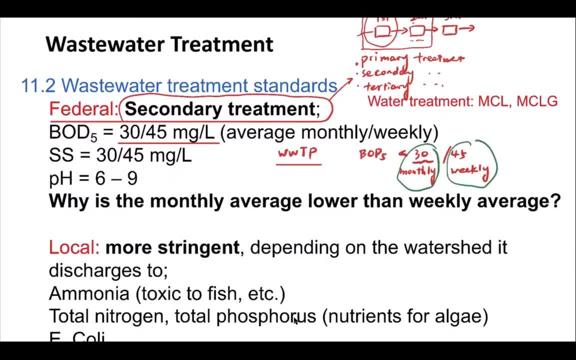 average. Why is it not the reverse? So this is our second quiz question, So I'm giving you a few options. So why do we have two different standards and why they are different from each other? So why they're not the same? 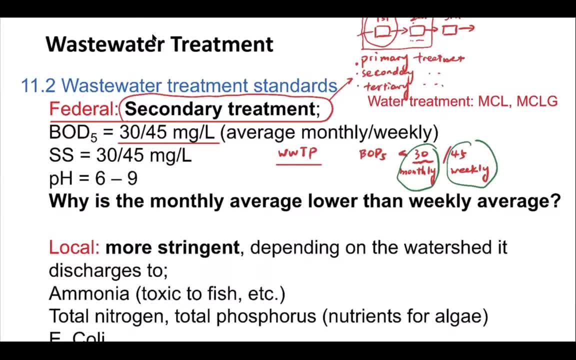 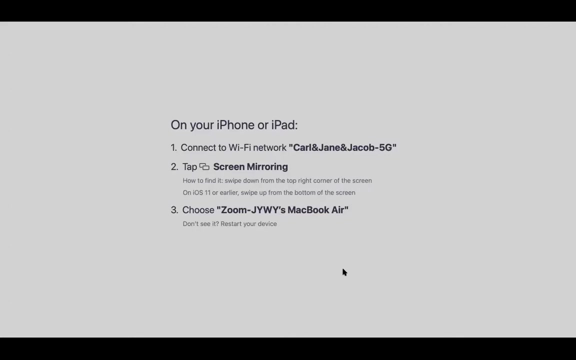 Okay, Five more seconds, All right. Okay, All right, All right, We'll stop here. So again, I think most of you get the correct answer right, So this is just to make sure that let's see. All right. So I think there may be some network problems. 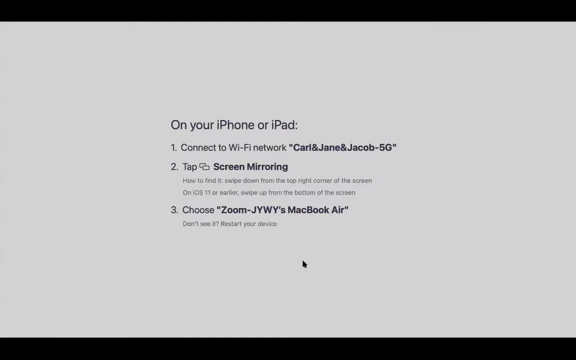 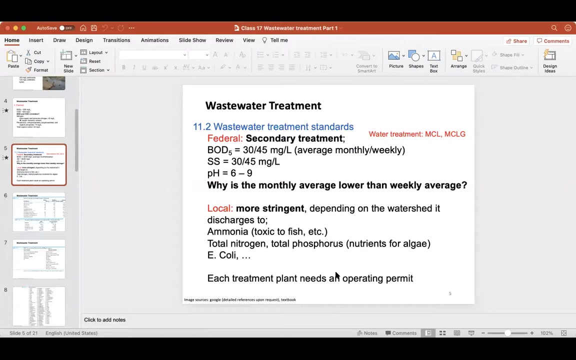 all right. So there may be some network problems. Let's just continue here. So I also have the powerpoint. may be we could just directly use that. Okay, So this is your answer. I'm just sharing the choice. I'm just a champion. This is the choice. You're my lucky day And then this is just an ichitet clear in-government. Yeah, All right, Okay. So one more question. So is it measures, PIPs, Metro sample, or is it PPI? That's for a interests? 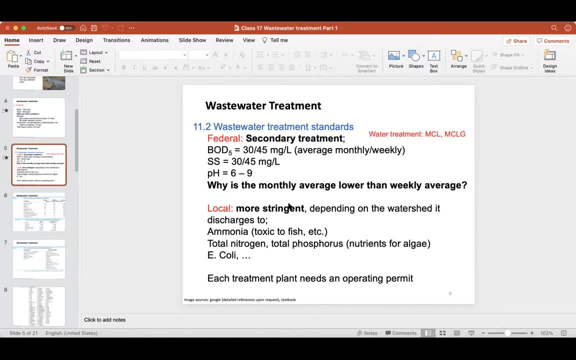 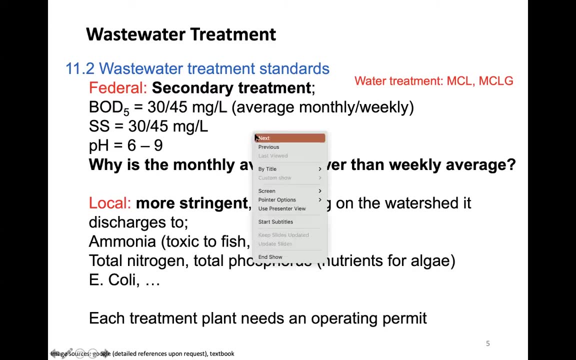 Okay, I'm going to ask a question now. Yeah, so basically, it's because of there are fluctuations in the contaminant discharge, right? so if we consider what is happening, so if we consider what is happening in terms of the discharge, let's say, if we plot the concentration of the contaminants as a function of time, right, so what's going to? 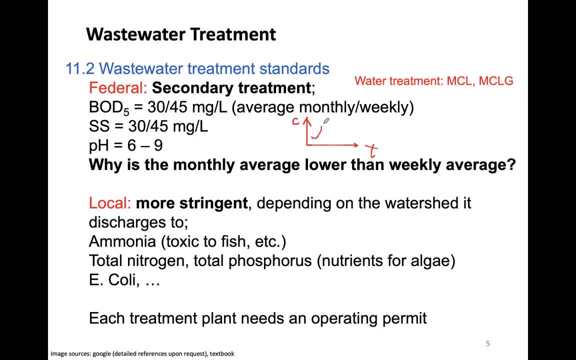 happen is we're going to have fluctuations. sometimes we can have very high concentration, sometimes very low concentration, right. so because of that, if we do the weekly average, then maybe we will conduct the measurement at this high concentrations here, right? but still, as long as the concentration is below 45, then we will have fluctuations in the discharge. 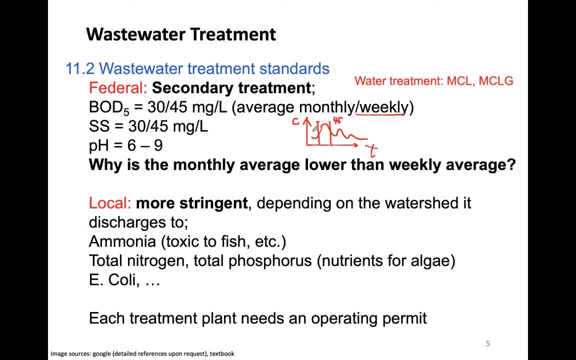 then we say that it's good, right, but in terms of the monthly average, what we're going to look at is the entire time periods, and we want to make sure that it is below a relatively low value so that it still satisfies the standard. all right. so this is the federal requirements, and we also 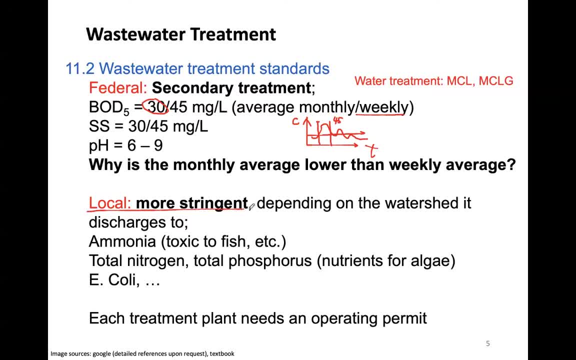 have the local requirements, so generally they're more stringent and it really depends on the watershed it's in right it's discharged to, because there are some ecosystems that are very fragile. so, for example, we want to limit the amount of ammonia because we don't want to kill the fish, right, the total nitrogen, so we don't want to cause any algae blooms, and also 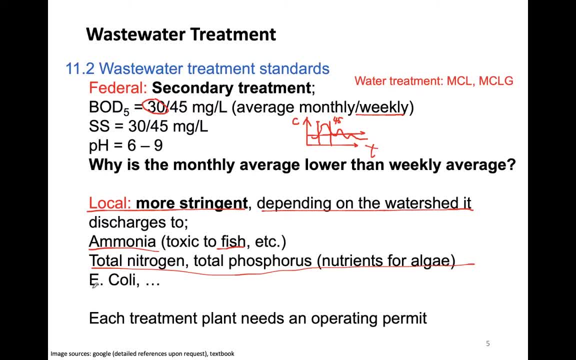 we don't basically want to control the amount of e coli because we don't want to harm the other, let's say the bacteria in the system- right, and also each treatment plant actually needs an operating permit, so we have to check what is the water quality and also they need to prove that they're 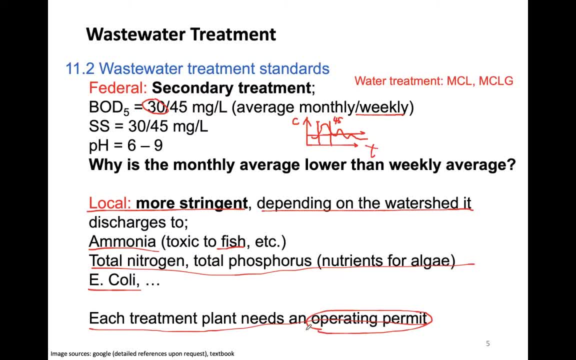 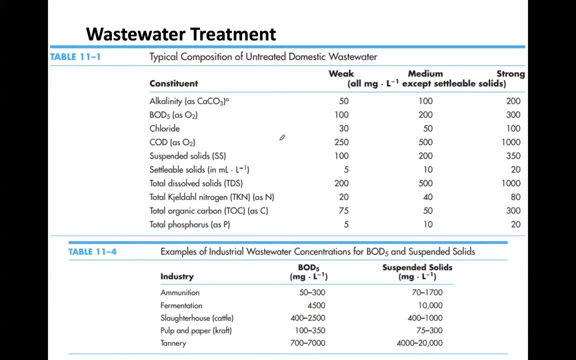 able to do these treatment processes because we don't want to accidentally spill the contaminants into the drinking water systems, right? so here, what i'm showing are actually a few tables regarding the wastewater quality. so, as we said, so there are weakly polluted or the lightly polluted, right the medium level of the pollutants, and 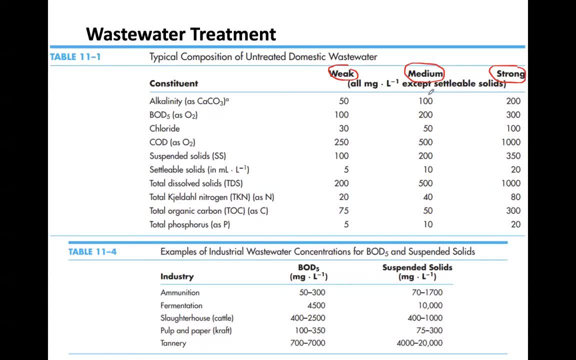 strongly polluted wastewater. so what i just showed earlier was the medium condition, okay. so actually people do a lot of measurements in terms of all the different, let's say, physical or chemical properties. let's say the alkalinity bod 5 chloride, cod suspended solids, right. so, for example, nitrogen here, right, carbon, phosphorus. so, as i said, the wastewater also strongly depends. 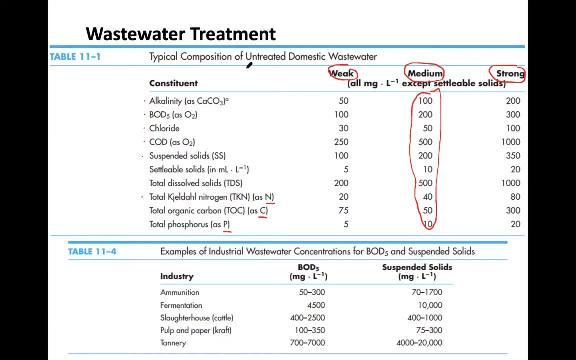 on the source from it, and this is mainly the domestic wastewater, so most of them are coming from the households, right? but in terms of the industry, it really depends on which industry we're talking about. so this is in dutch industrial wastewater concentrations, so it's listing a few. 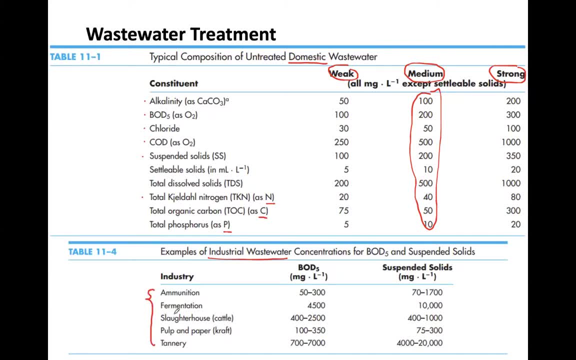 industries. so we can have the ammunition, fermentation, slaughterhouse, pop and paper and tannery right where people make leather right. so you can see that the slaughterhouse and the tannery they can have very high bod values, mainly because we're dealing with meat right, so meat is full of. 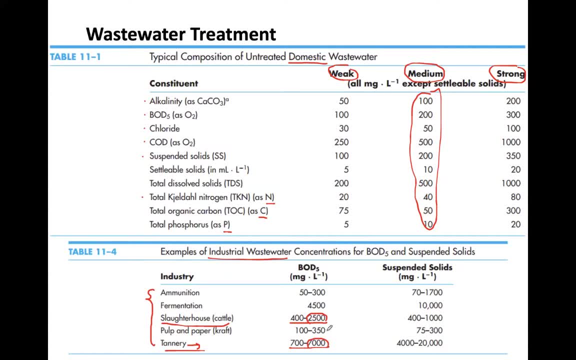 organics, we have to dump it into the wastewater treatment or the wastewater stream and fermentation is pretty high as well. but in terms of the problem paper um, the bods are relatively low right, and because of that for different industry they can use some pre-treatment to deal with the bod5 or and 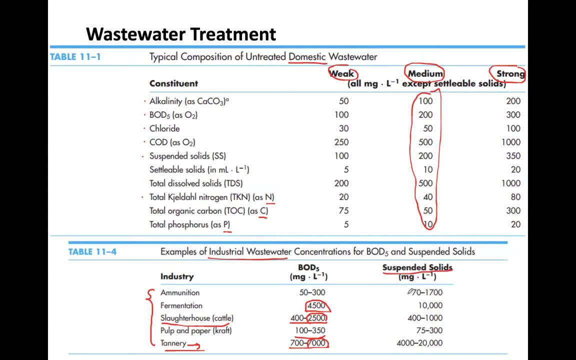 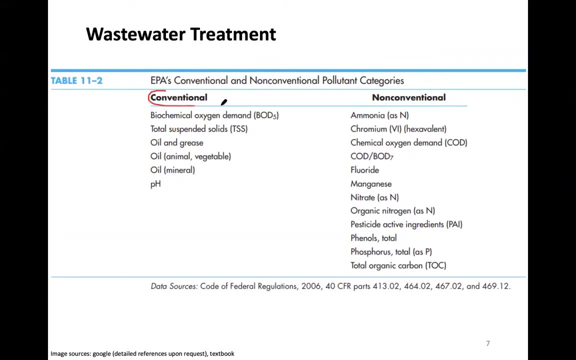 also the suspended solids, before they discharge them into the uh, the wastewater treatment plant. so this is going to do a big favor for the wastewater treatment plant. okay, so, um, so here, um, i'm going to start by listing some conventional uh pollutant types and non-conventional pollutant. 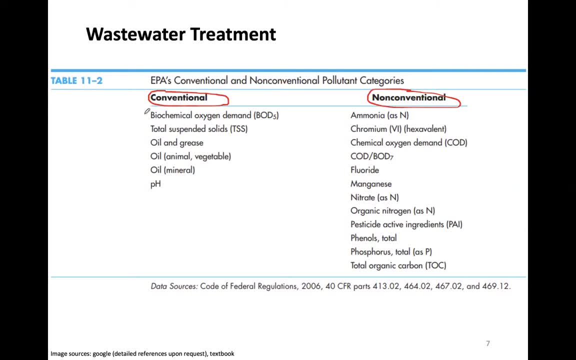 types, right, so the conventional pollutant species are those that we're most interested in. people have been doing this measurement for a long time. right? for example, bod5, suspended solids, ph and different types of oil. in terms of non-conventional, conventional pollutants, then they're going to be. 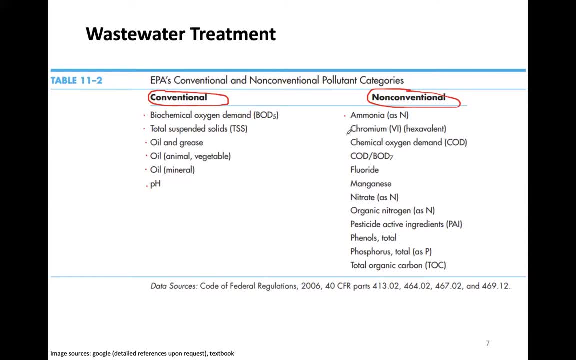 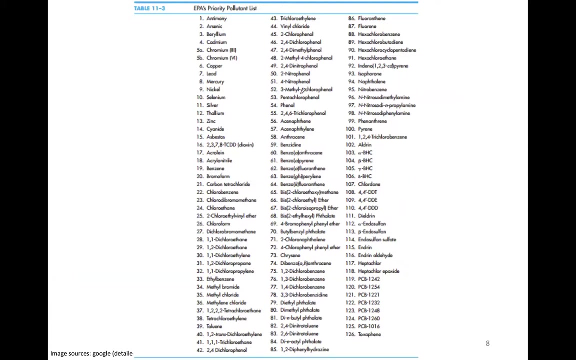 more detailed quantification of the physical and chemical species, let's say ammonia, chromium cod, let's say fluoride nitrate. so they're going to be more detailed measurements here. but actually epa has done a very good job defining all the pollutants that may exist in the wastewater. so you can see that there are 126 of them. so people can. 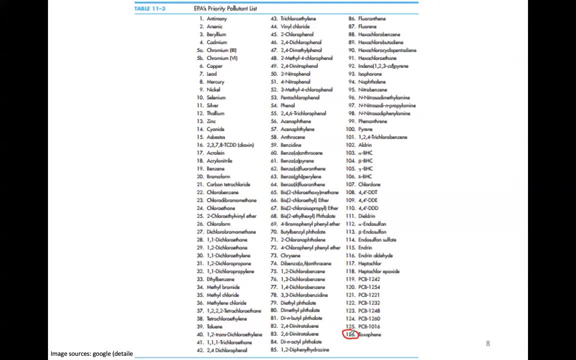 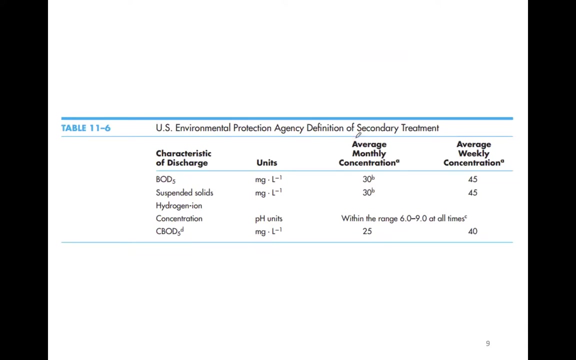 do these measurements to make sure that the wastewater that discharge back into the environment, they satisfy the water quality right: we don't have a, let's say, a very high concentration of mercury when you discharge them back into the environment. so, finally, this is the again the epa established instrument established limits in terms of the 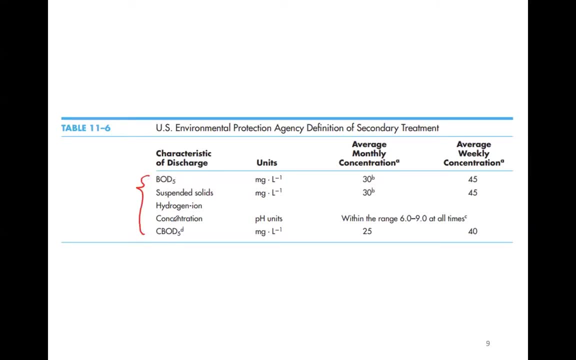 different types of contaminants: bod5, suspended solids, hydrogen ion. so basically this is the ph right and the cbod. again you can see that the monthly average is lower than the weekly average. so it is actually quite easy to, let's say, memorize the number right, at least for the 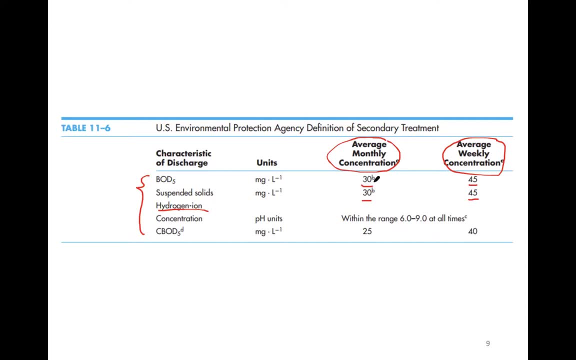 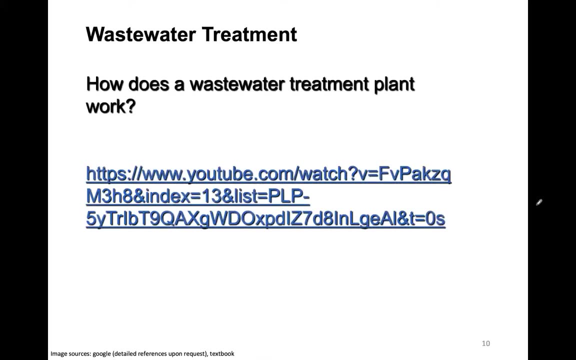 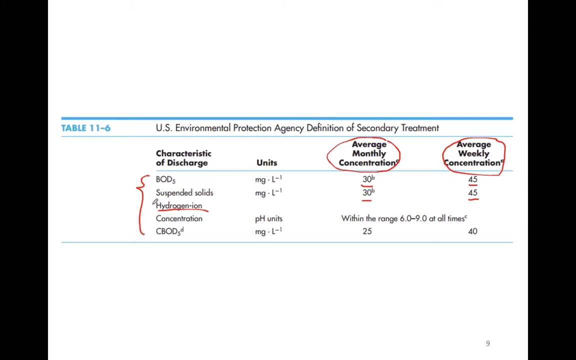 bod5 and suspended solids. they have the same number here, one is 30 and the other is 45. okay, um, so now we have the standard right, we know that this water is very polluted, right, and at the same time, the epa has, i would say, pretty stringent standard because, if you recall, 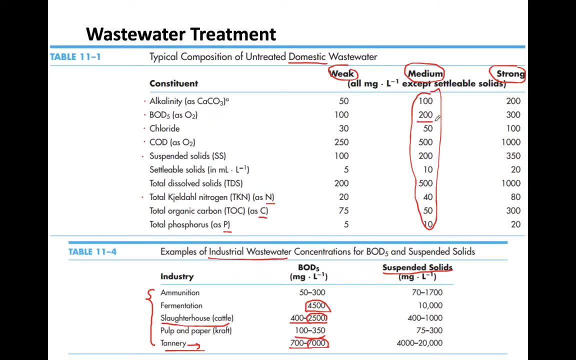 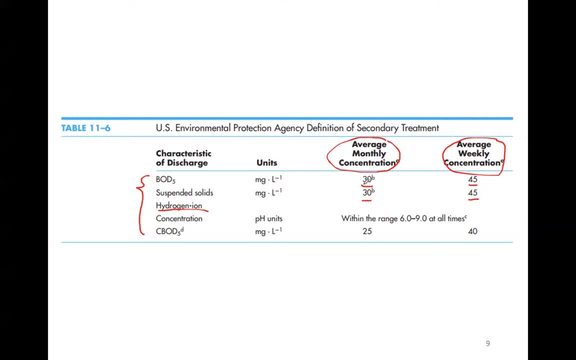 earlier in this table. so this is what the bod5 looks like: right, 200, and the target is 30. right, which means that we have to do a lot to get rid of the bod and also the suspended solids. right, so this involves the design of the wastewater treatment. okay, so how does the 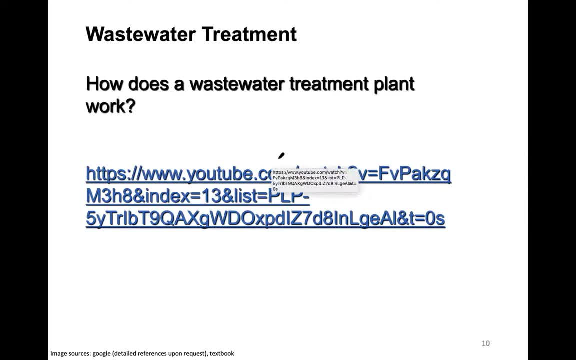 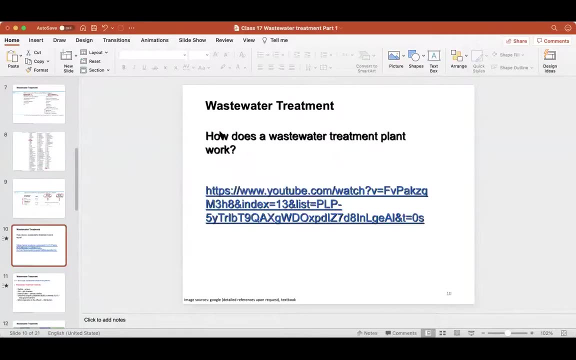 wastewater treatment plant work. so before i talk about the details of the- let's say the details of the wastewater treatment plant, i think it's good that we can go over a video first. right, it's going to be quite helpful. let's keep it and then just share this. 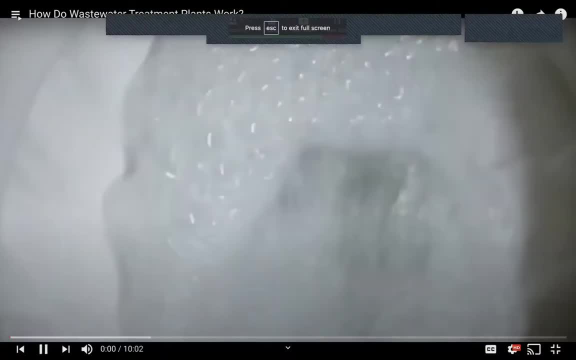 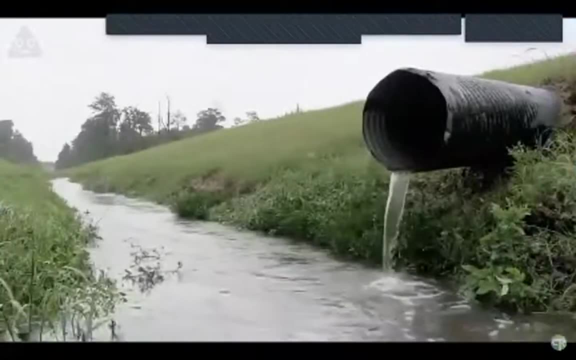 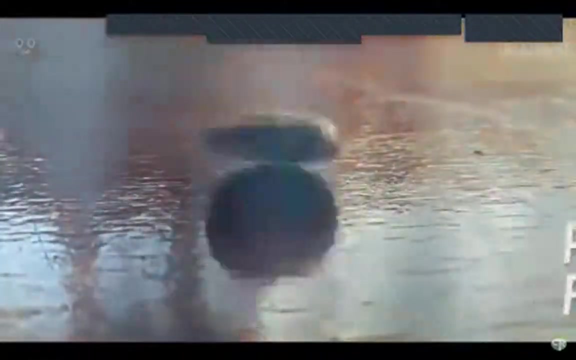 okay, here it is. it's a topic we'd rather not think about. where does last night's dinner go when we flush it down the drain? well, you may already be grossed out just thinking about it. this question leads way to a significant subset of civil engineering and a massive amount of public funding, just like all. 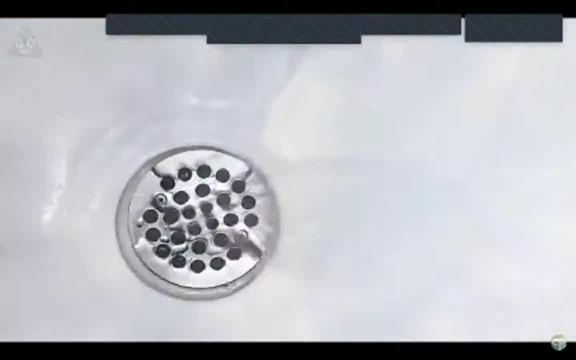 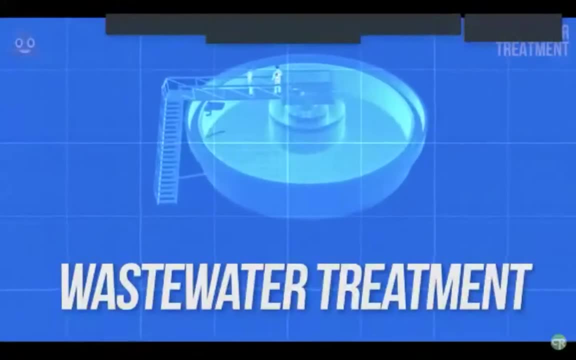 dogs go to heaven. all drains in the city lead to a waste of water, to a wastewater treatment plant where that wastewater gets turned back into water that we can drink. Now you may be thinking that you'd rather just let bygones be bygones and not think. 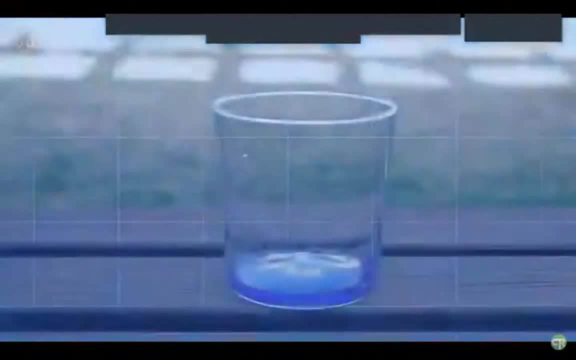 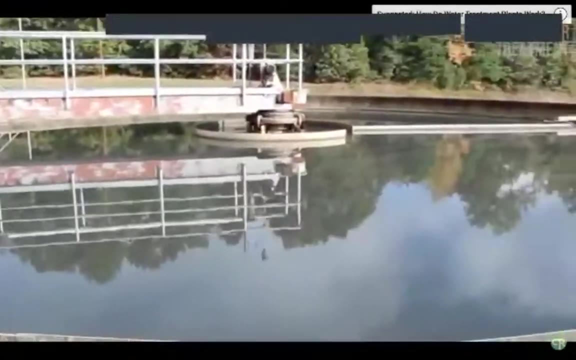 about this nasty part of real life. But here's the thing. Chances are, you've drunk water that was waste at some point, so you might want to take some time to understand this engineering process that makes dirty water clean. Here's where it starts The toilet Once you're done doing your. 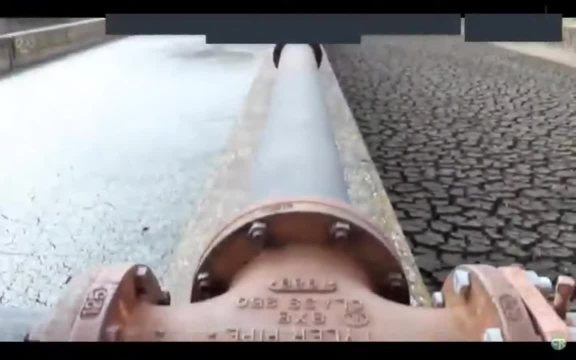 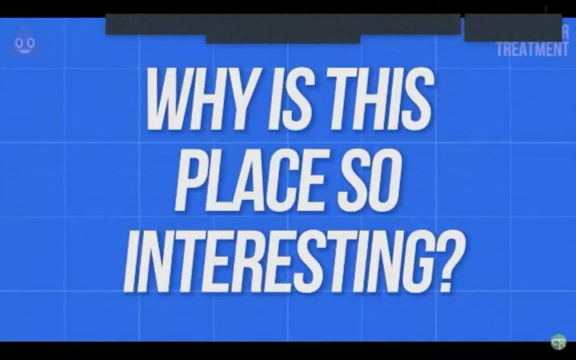 business and flush that magical handle, your waste ends up at the inlet of one pretty interesting place, a wastewater treatment plant. Why is this place so interesting? Because it takes arguably one of the most disgusting substances in the world and turns it back into something that is. 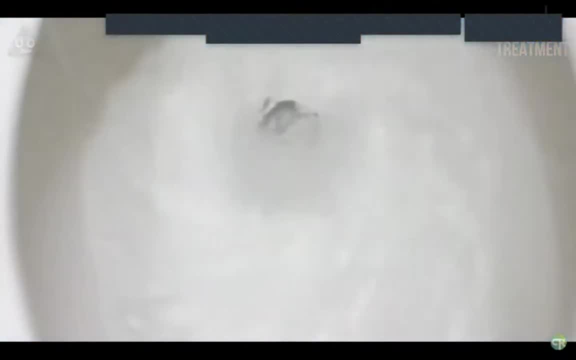 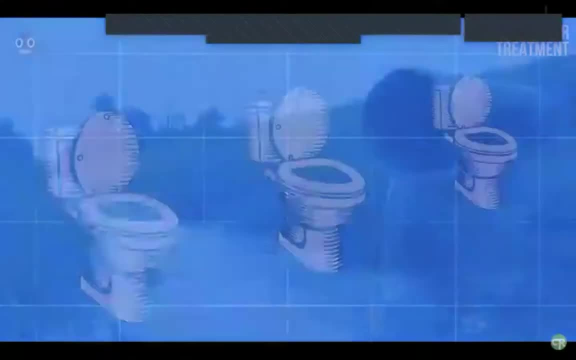 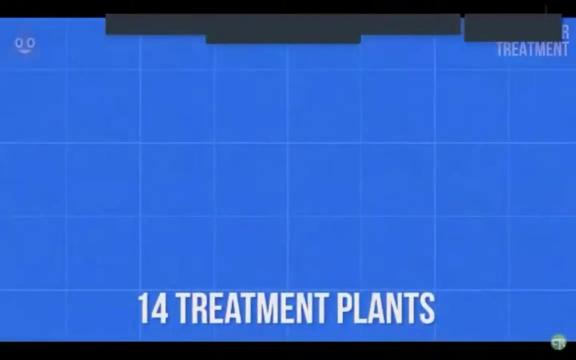 essential to all life. Flushing just your toilet at halftime may not seem like a big deal, but when you couple it with thousands, if not millions, of others doing the same, it can result in some pretty high sewage flow rates. The city has an array of 14 wastewater treatment plants that handle a combined 1.3 billion gallons. 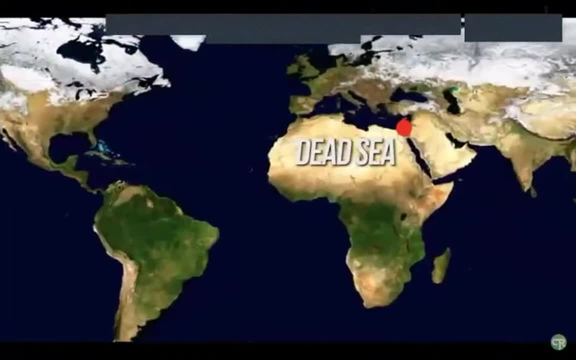 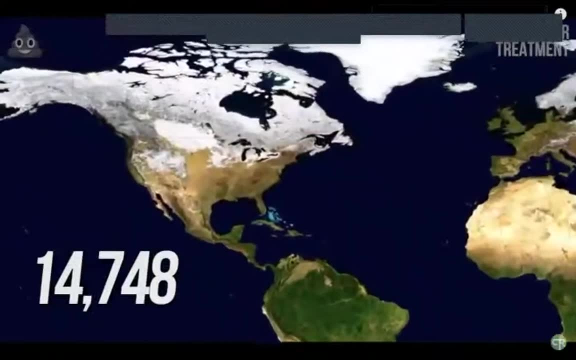 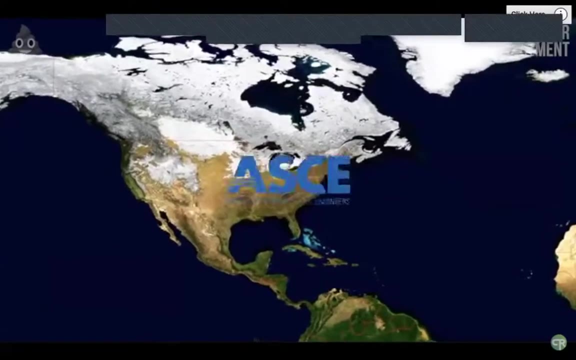 of wastewater daily. That's enough wastewater to fill the Dead Sea with pure sewage in just eight years. And that's just New York City. There are an estimated 14,748 treatment plants in the US alone that 76% of the USA's population relies on, according to the American Society of Civil. 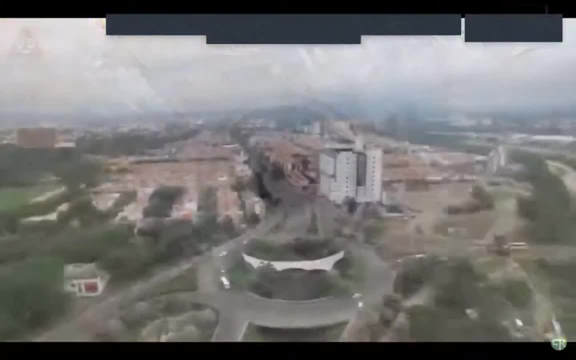 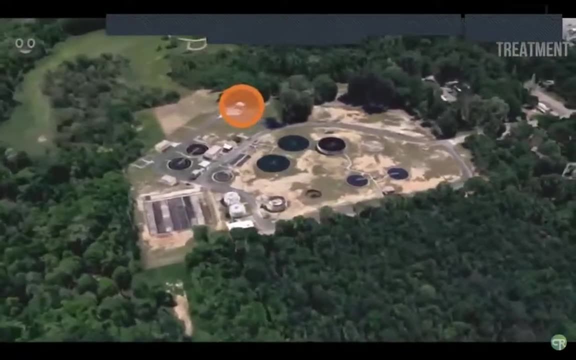 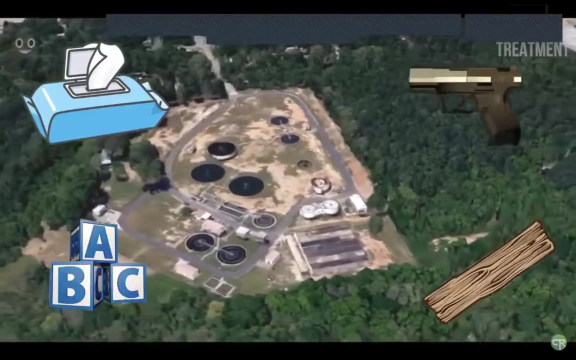 Engineers. Understanding wastewater is crucial to understanding the critical infrastructure needed to support modern life. That brings us to the first step of the process that handles larger items in sewage, things like flushable wipes, 2x4s, toys or even guns- You name it, and it's probably 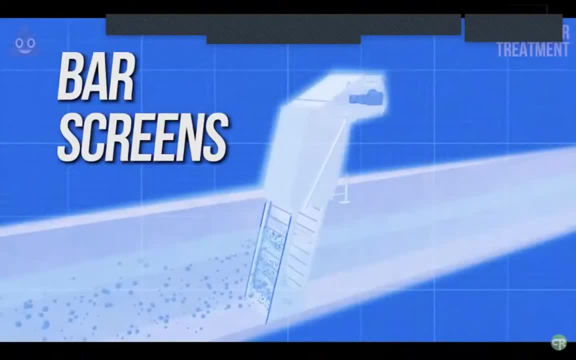 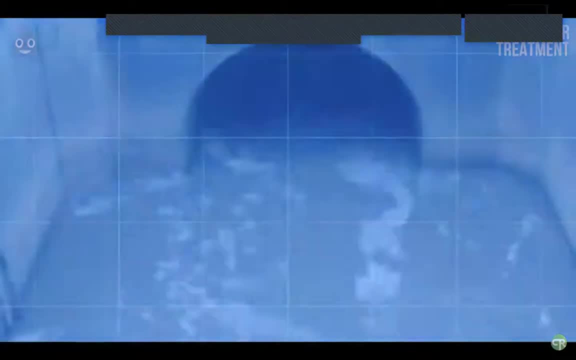 been caught in a bar screen. Bar screens are exactly what you would think. They are large vertical bars that stand at the inlet of nearly every wastewater treatment plant, designed to stop larger items from getting to the plant and hurting machinery like pumps. This first process. 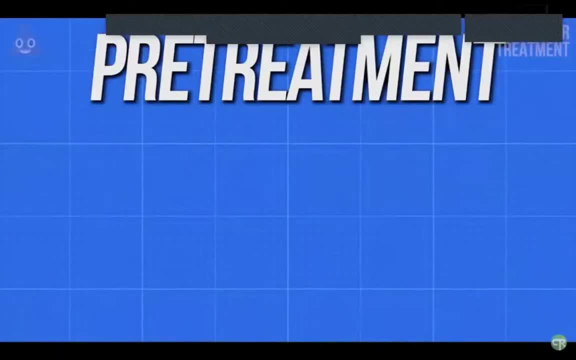 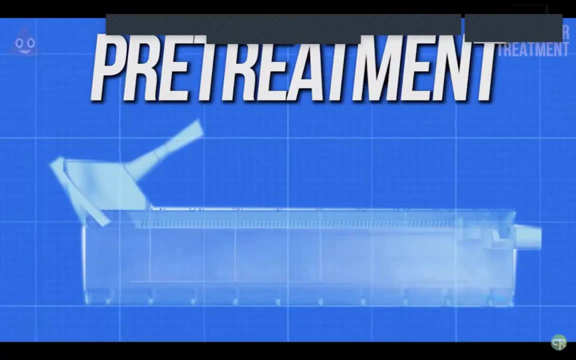 is commonly referred to as pretreatment. The sole intention of pretreatment is to remove the outliers in the sewage and make the whole mixture a little more homogenous or slightly less chunky. Bar screens are typically mechanically raked at certain intervals, depending upon 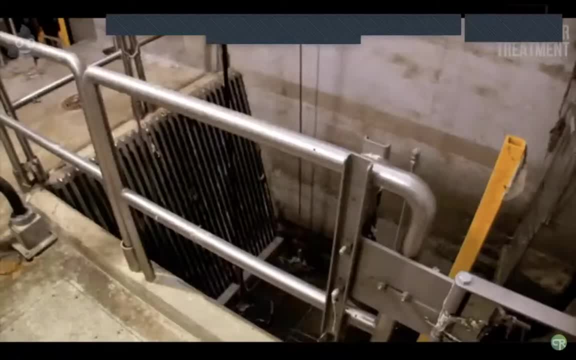 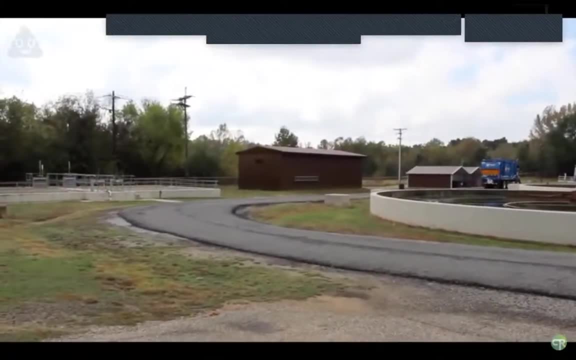 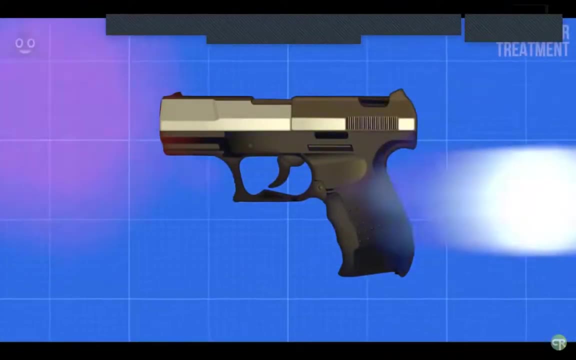 the flow rates of the water treatment plant, although some older plants will still have more manual removal processes. Whatever is removed from the bar screens is then sent off to your average landfill or solid waste handling facility Or, in the case of unusual items such as guns, they are sent off to the evidence locker in a police station to. 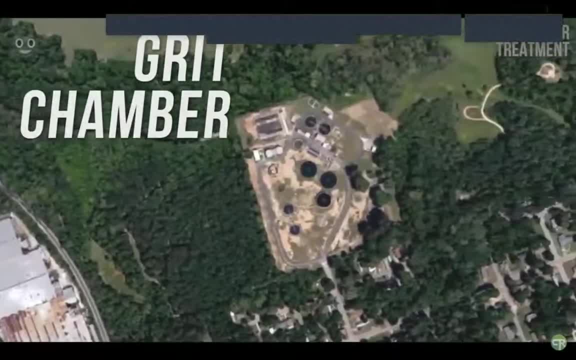 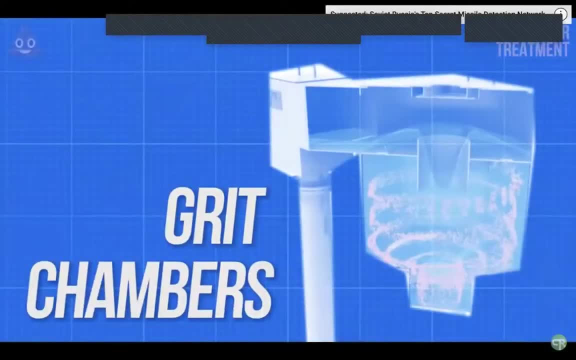 be investigated. Next up is the grit chamber. Grit chambers are the next steps in the pretreatment process following bar screens. Since these bars don't catch everything, larger particles called grit still need to be removed from the sewage as it is made even more homogenous As the 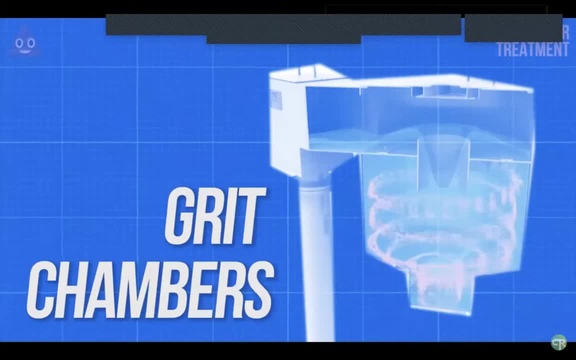 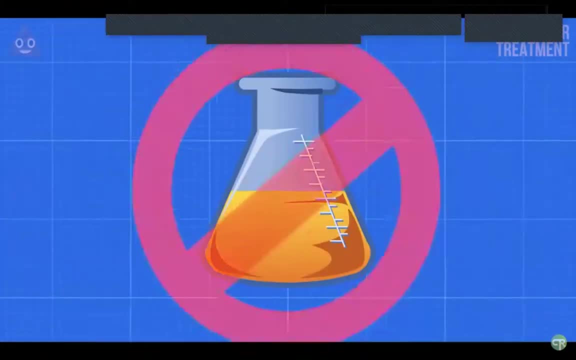 sewage flows into the grit chamber, the velocity of the rather viscous sewage is adjusted to allow for particles of sand and rock to settle out. This is needed because these particles can't be removed using chemicals and they could potentially clog or destroy pumps later. 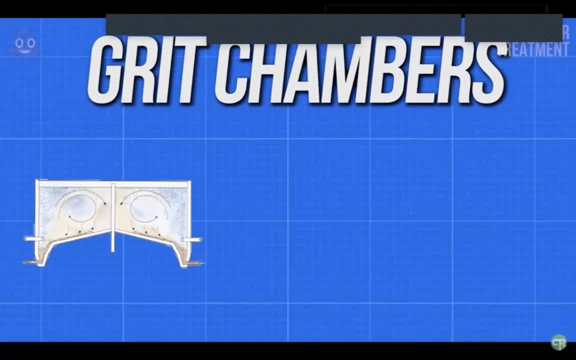 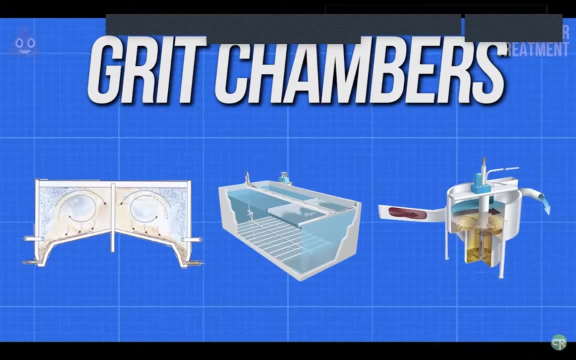 on in the process. There are three types of these chambers: horizontal grit chambers, aerated grit chambers and vortex grit chambers, which all accomplish the same task using slightly different methods. Following the grit chambers, the sewage will move onto the primary treatment. 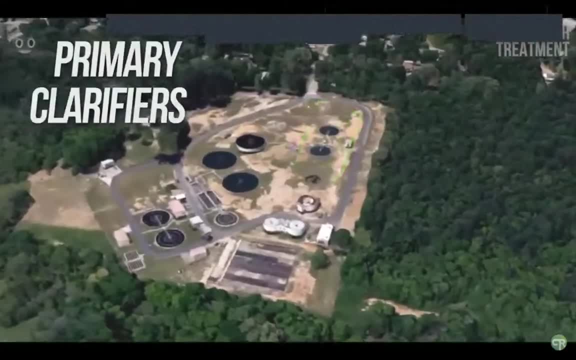 process which starts with a large basin called a primary clarifier. Primary clarifiers and clarifiers in general function on the principle of settling velocity. The primary clarifier is the primary clarifier that is used to determine the velocity of the sewage. The primary clarifier. 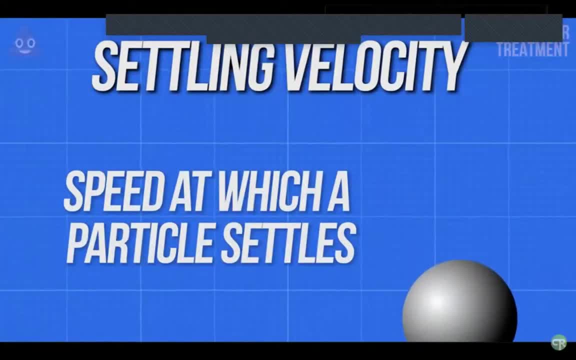 in general is the primary clarifier that is used to determine the velocity of the sewage. This term can be defined simply as the speed at which a particle settles For wastewater being pumped into clarifiers. it's important that the flow rate of the water being pumped 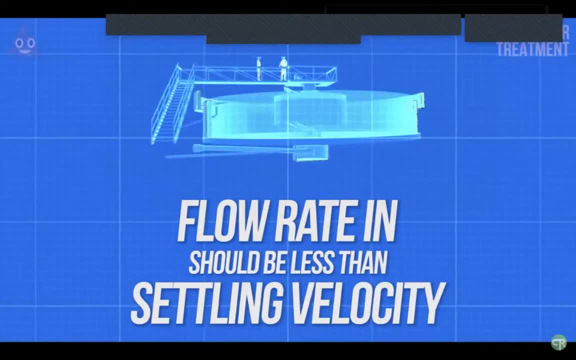 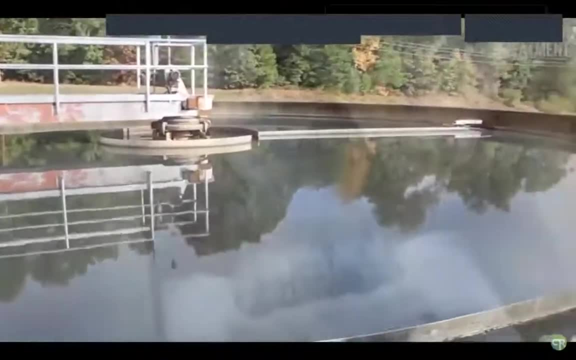 in doesn't exceed the settling velocity of the particles trying to be removed. In order to accomplish this, engineers will vary the size and number of primary clarifiers in accordance with the plant's permitted sewage flow rate. This ensures that at varying flow levels, 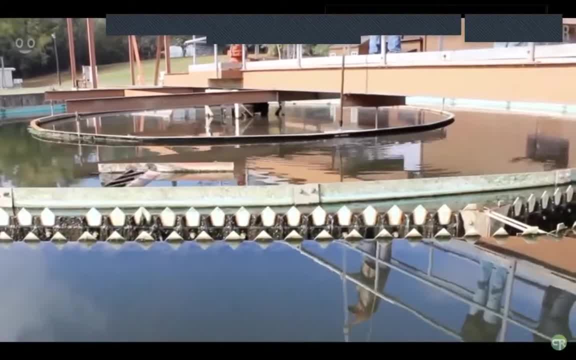 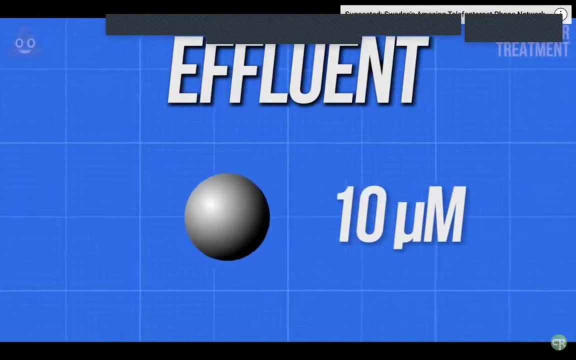 solids can settle out of primary clarifiers to the correct quantities At this step in the process. the slightly treated wastewater, which is referred to as effluent, is free of solids larger than 10 micrometers and should be all organic matter which will be treated. 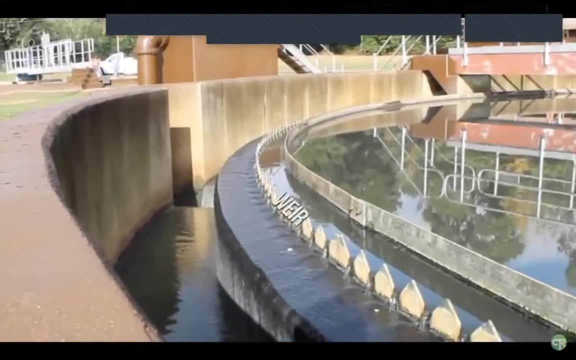 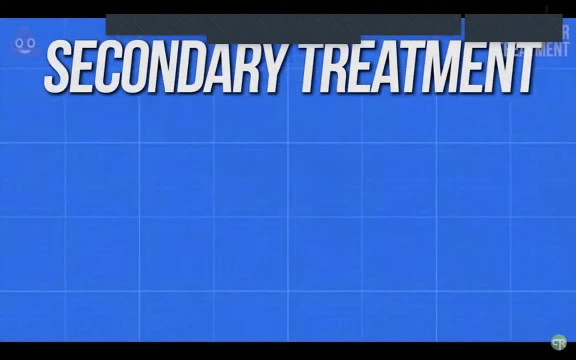 further. The top layer of the clarified water flows over a weir wall and into the next basin in the process called the aeration basin. Now begins the process of secondary treatment, the sole focus of which is to significantly degrade the biological content of the sewage. 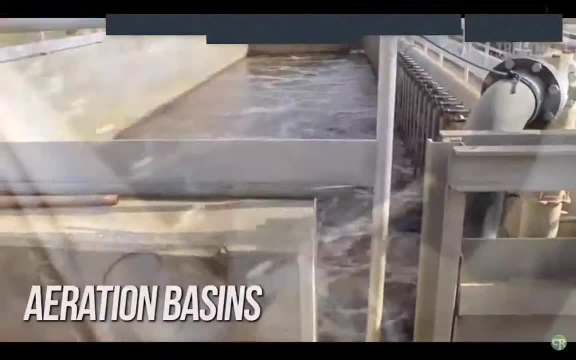 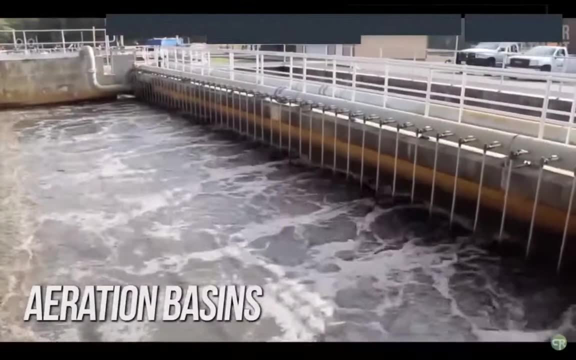 In many cases, this process starts with aeration basins. Water flows into the aeration basins, at the bottom of which are hundreds, if not thousands, of tiny air blowers that create bubbles through the water. The water is pumped into this tank. 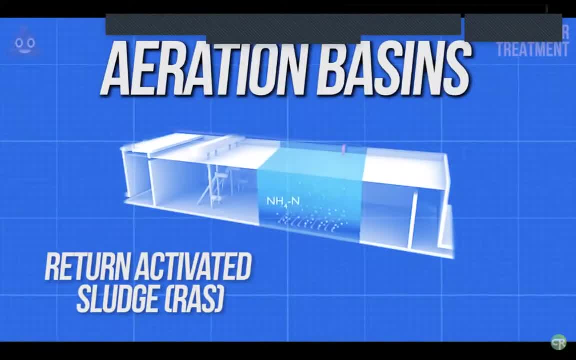 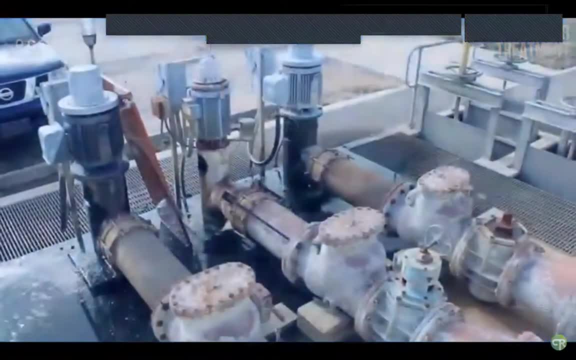 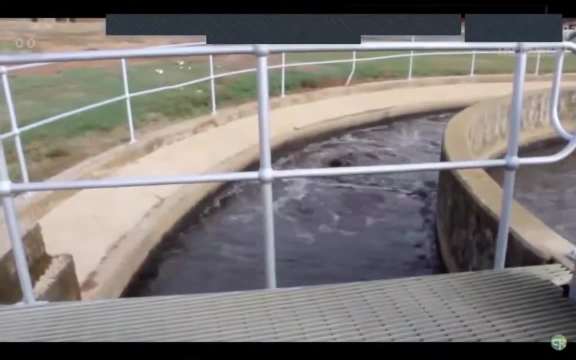 along with something called return-activated sludge. You can think of return-activated sludge as a bunch of happy little bacteria that get to eat their favorite foods all day long. This introduction of significant amounts of bacteria, along with the massive amounts of oxygen injected from the bubblers, creates an environment perfect for the process of. 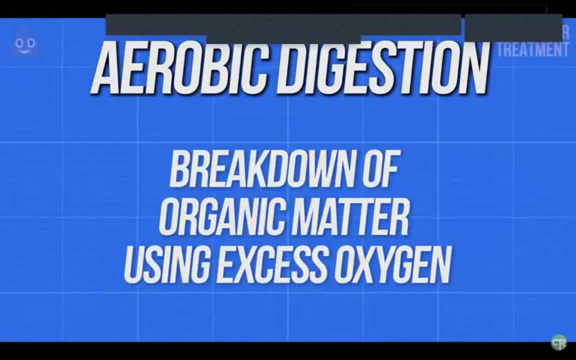 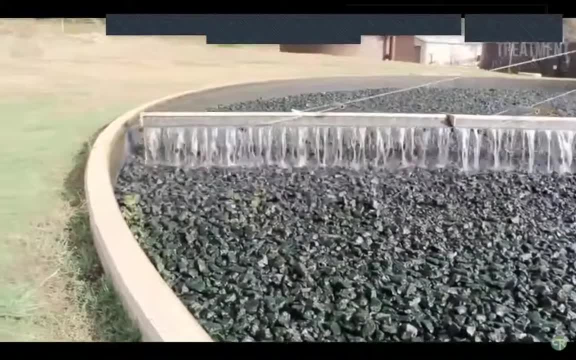 aerobic digestion. Simply, it's the breakdown of organic matter along with the use of excess oxygen. Some older plants will add in another step before aeration basins referred to as biofilters or trickling filters, Found in many older plants. these filters essentially trickle. 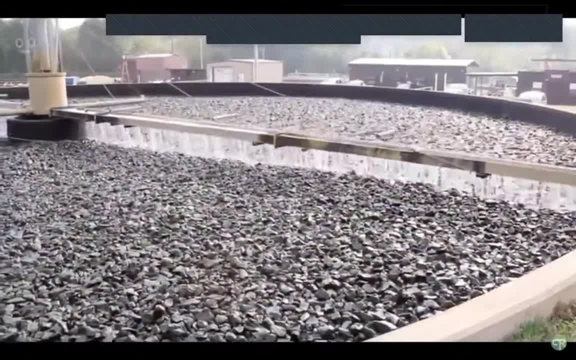 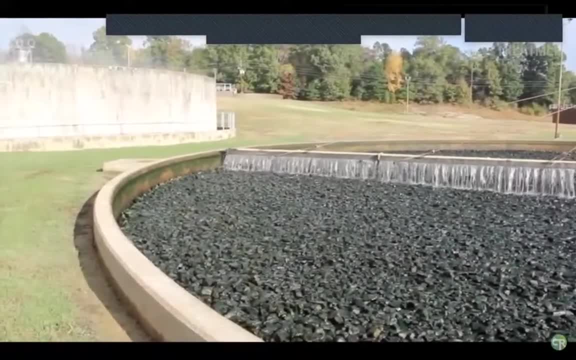 the effluent over a medium like stone or plastic and allow for a film of bacteria to chow down on any organic matter in the water. This step is largely not used in newer plants due to more efficient and effective modern processes, But for plants with basins already installed. 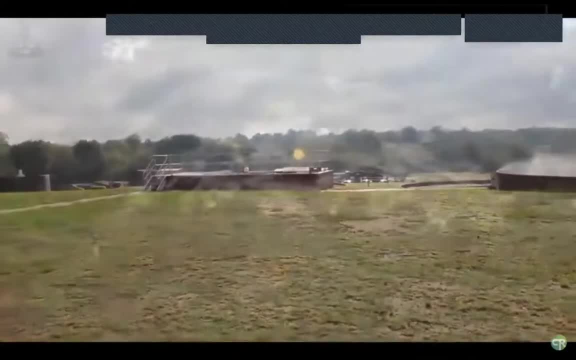 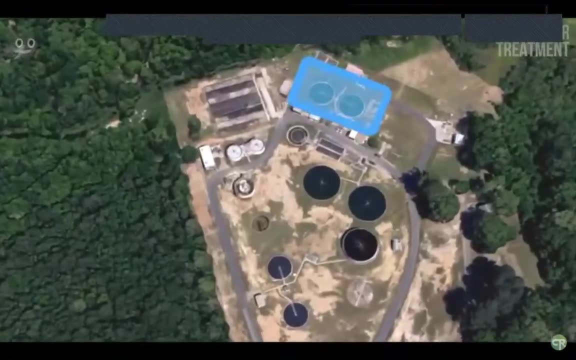 they still use them because they only benefit the treatment process. in most cases, Following aeration basins, the effluent, along with much of the sludge, is pumped into a secondary filter or clarifier, where some of the sludge is removed and pumped back into the aeration. 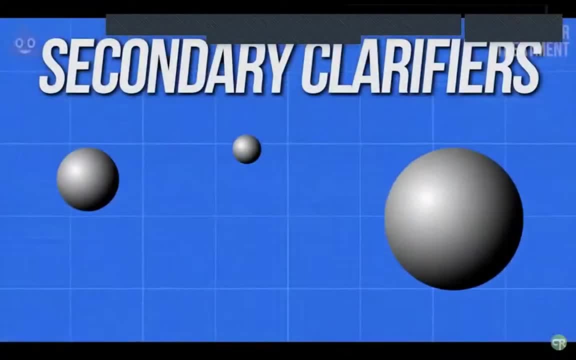 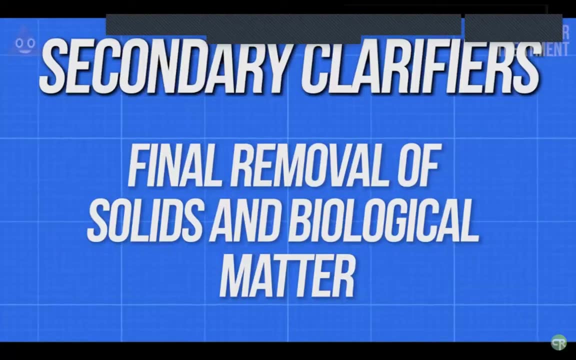 basins as the return-activated sludge. Further settling of larger particles is also accomplished in these basins, as it is the final step of the process that will remove solids and larger biological matter. Water flows out of secondary clarifiers over a nearly identical weir room. 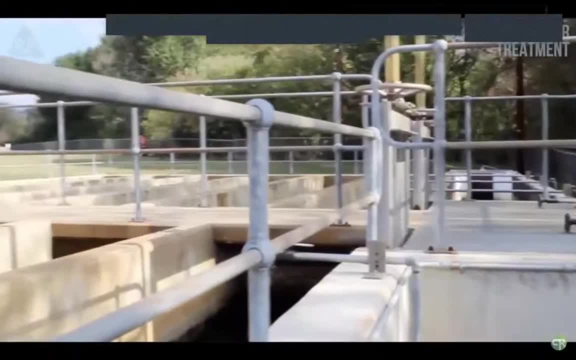 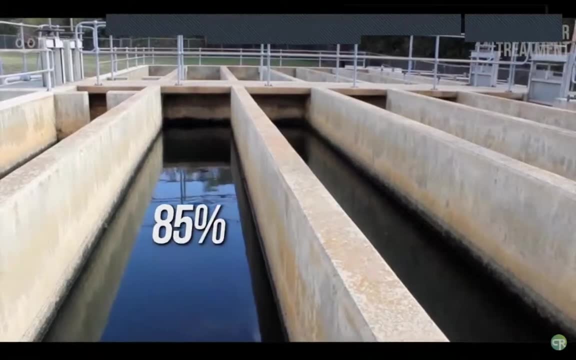 the weir wall to the primary clarifiers and moves on to the disinfection process. At this point, 85% of all organic matter is removed from the water and the effluent should be safe to drink in most cases, although you probably wouldn't want to. 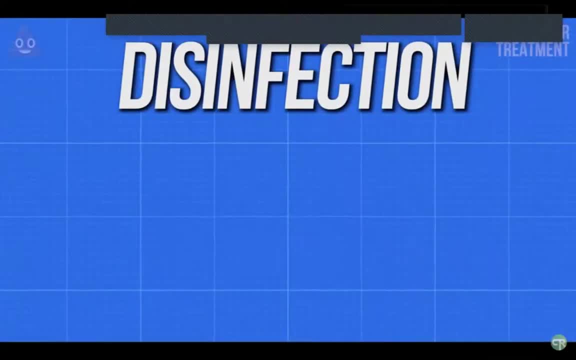 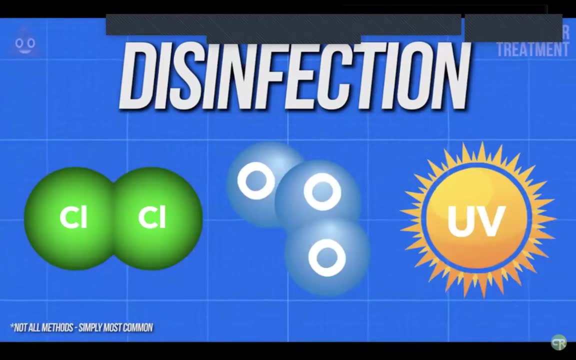 Disinfection is the final step of the process and is usually accomplished in one of three ways, either through chlorine ozone or ultraviolet disinfection. Each process has its benefits and drawbacks, with each being used commonly throughout the wastewater treatment process. 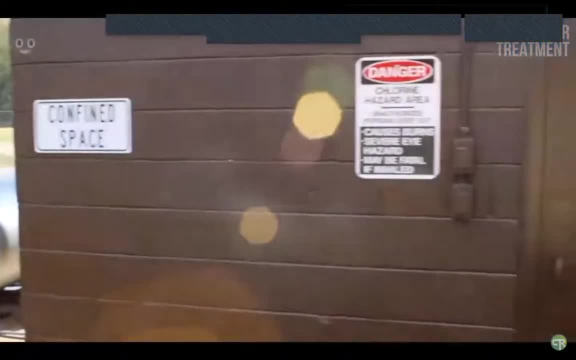 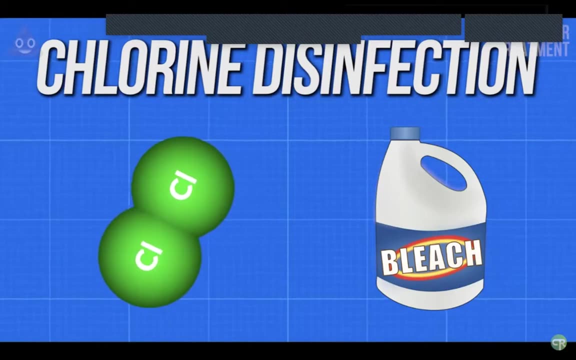 Chlorine disinfects the water through chemical disinfection. Chlorine, which you can think of as concentrated bleach, is added to the effluent here to kill off any remaining bacteria and organisms still living in the water. When chlorine is added to kill off the bacteria, 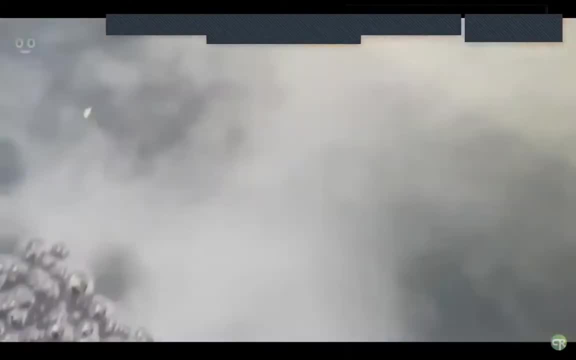 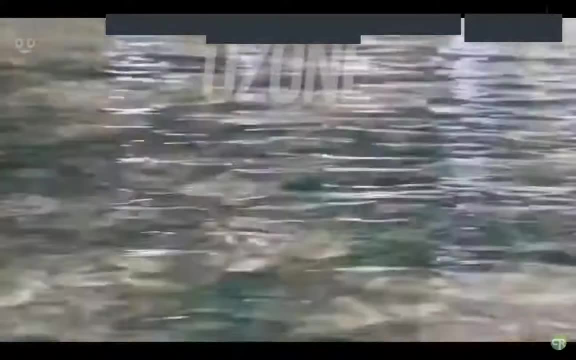 it then has to be removed before it can be discharged, as to not kill off anything in the discharge location. After this, the water is safe enough to discharge into a stream or lake. Ozone disinfection is another method of disinfection that is used to disinfect water. Chlorine is. 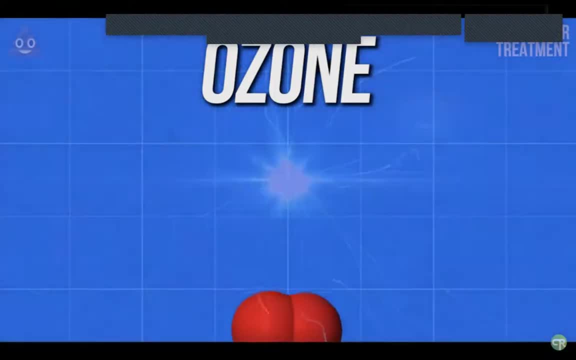 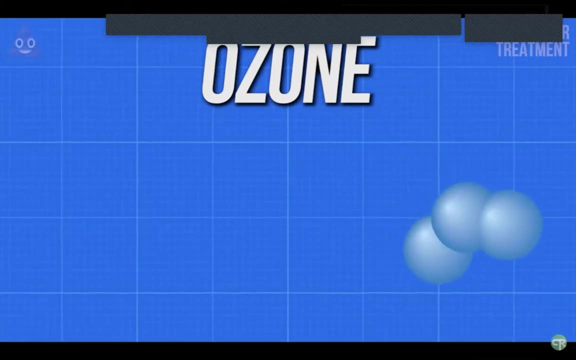 the first method that involves pumping an electrical current through the water that causes oxygen molecules to disassociate and combine with a free oxygen molecule, forming O3, known as ozone. Ozone is an incredibly strong oxidant and causes microbes' cell walls to leak. 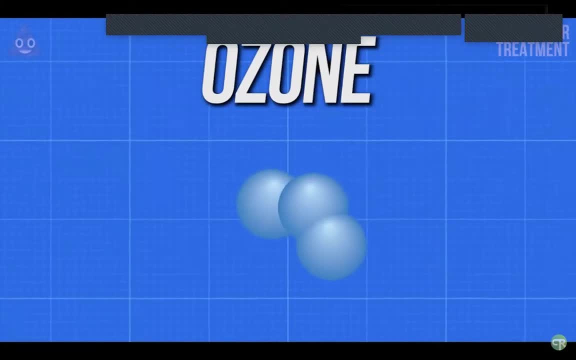 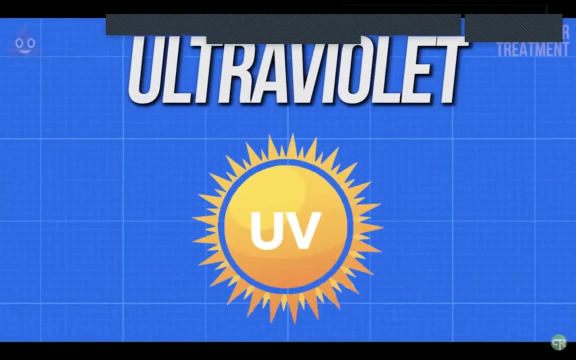 rapid cell decomposition and overall damage to cells. In other words, it kills off bacteria. The last common method uses ultraviolet light to scramble bacteria's DNA so that they cannot multiply. In UV disinfection, the bacteria can be removed from the water by pumping an electrical current. 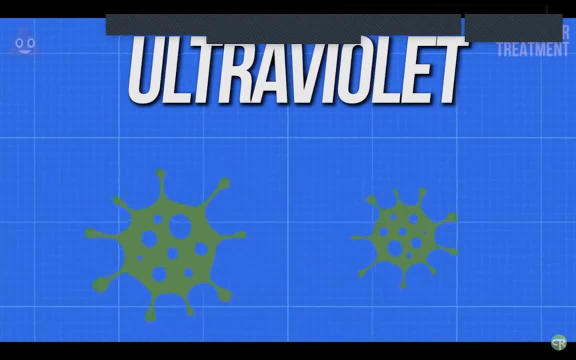 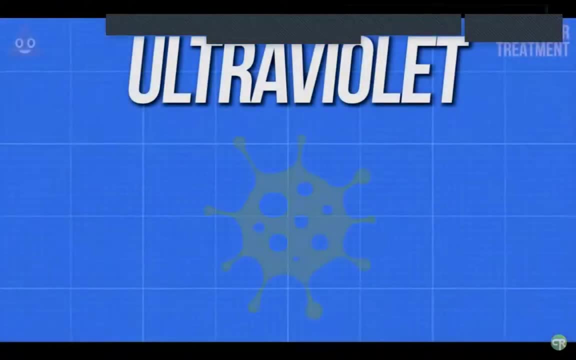 into the water. The bacteria in the water aren't killed. rather, they're sterilized, rendering them harmless. If you were to ingest water with living microbes immediately following UV treatment, any harmful bacteria would be unable to multiply or render your body damage. 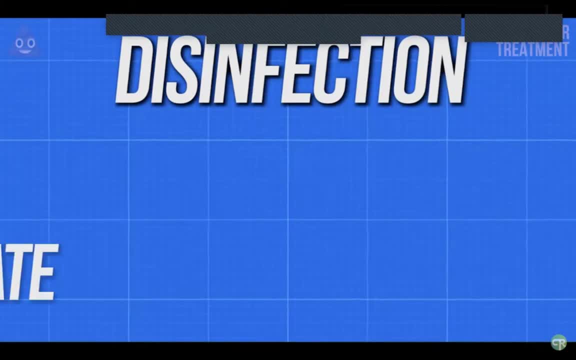 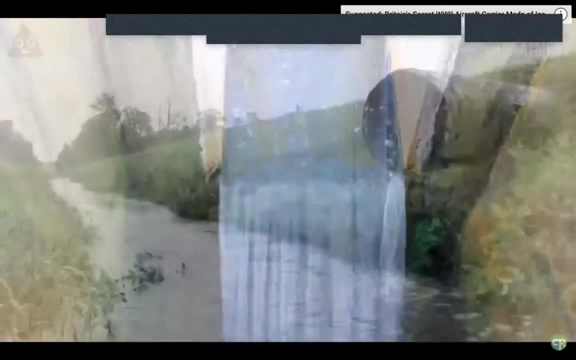 Engineers choose between these methods based on a variety of factors such as flow rates, cost and location of discharge, which brings us to the final step: effluent release. Effluent release exists in one of two forms. In most cases, the now-treated water is very. 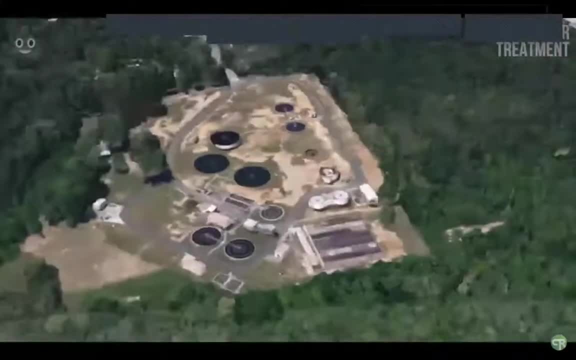 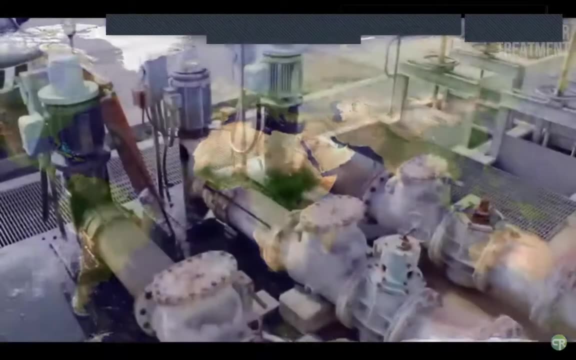 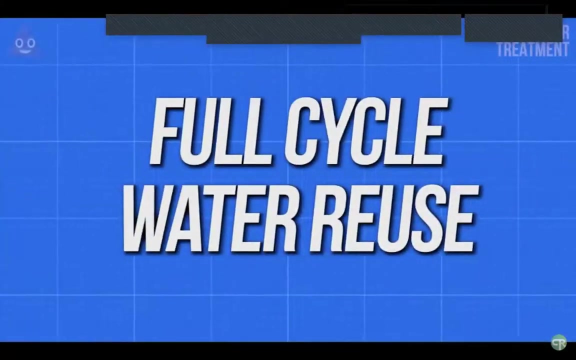 easily released back into a stream or lake or other water source. In rare cases, usually in areas where water is scarce, the effluent discharge from a wastewater treatment plant can be discharged into another treatment plant directly, where it will be treated further for consumption. This is referred to as full-cycle water reuse From a chemical perspective. 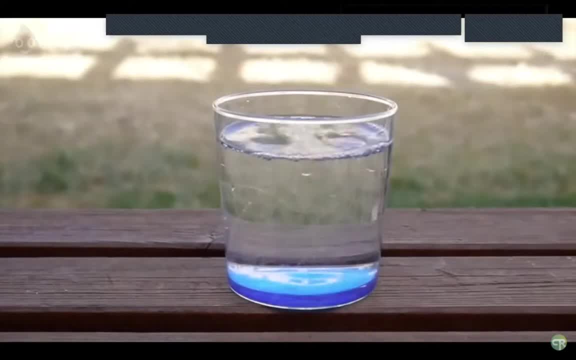 the final drinking water is the same as normal treated water that flows through your pipes now, but due to the connotation of your drinking water being sewage just days before, this treatment process is not as effective as it used to be in the first place. This process, 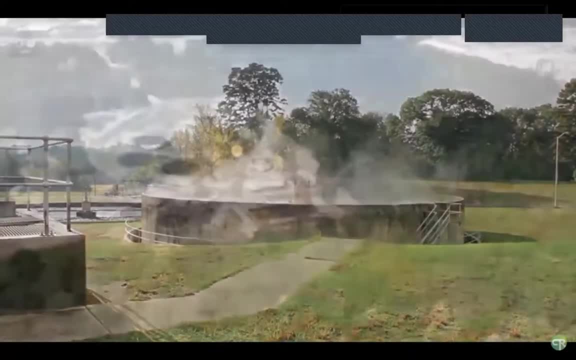 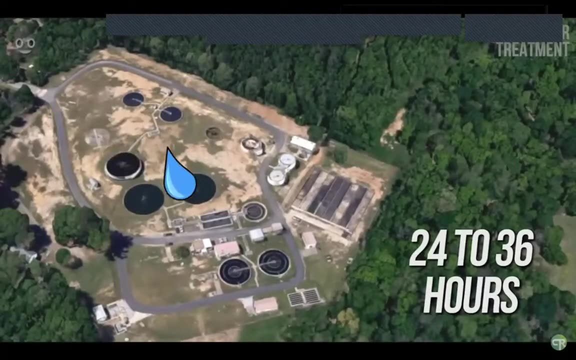 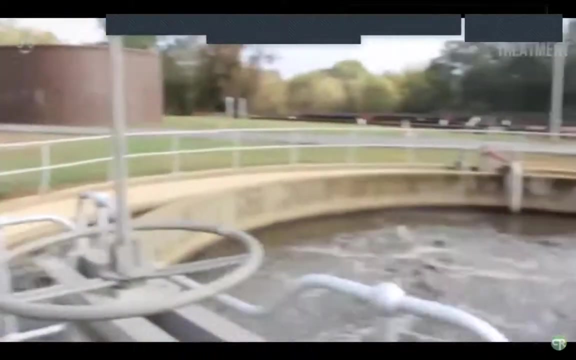 is normally shied away from or not heavily publicized. The entire process of wastewater treatment takes, on average, 24-36 hours from when a drop of water enters to when it leaves. Each wastewater plant will receive a permit for flow rates, chemical levels and effluent quality, among other things, from the EPA. 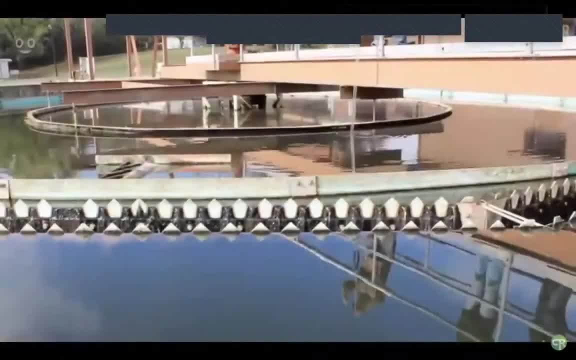 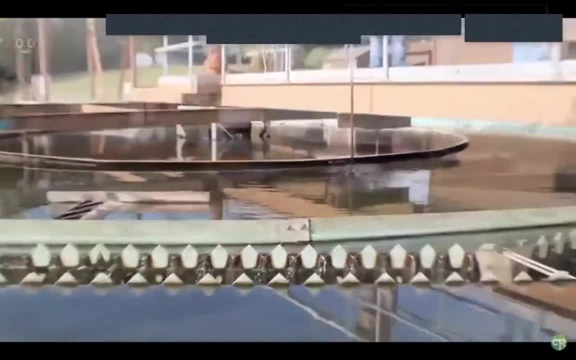 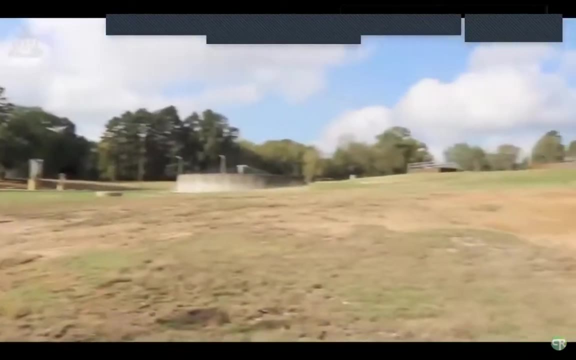 that outlines the necessary treatment for a plant Wastewater plant. operators will make adjustments to a plant's operation and constantly measure levels to ensure proper discharge and proper treatment. Without these operators and the dirty job that they do around the clock, our sewage would always stay sewage, and sanitation in modern cities would be much, much worse. 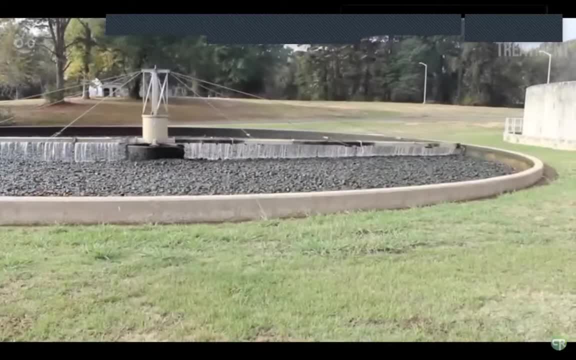 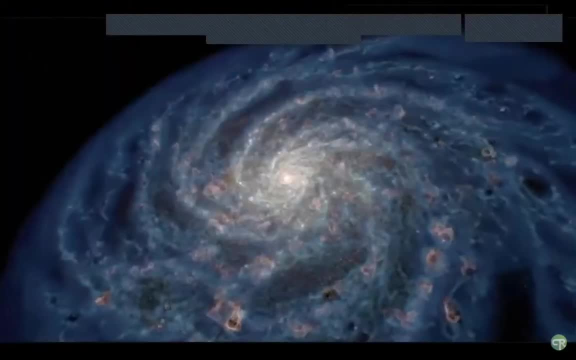 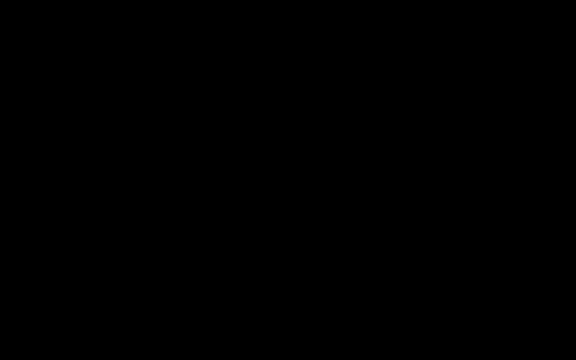 Wastewater treatment is an essential dirty job, and you can thank the 14,748 treatment plants in the US alone for not having to worry about what happens when you flush. Okay, so I think this is a very nice overview of the 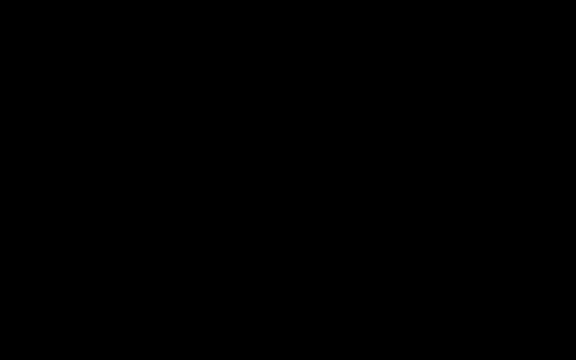 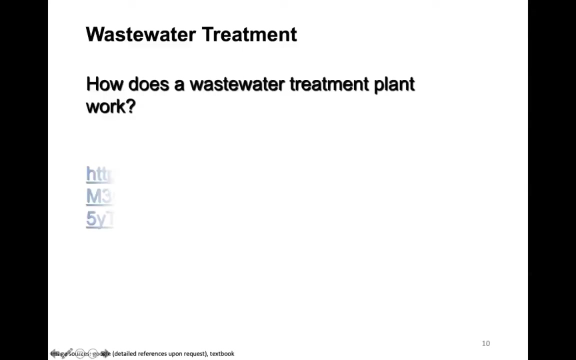 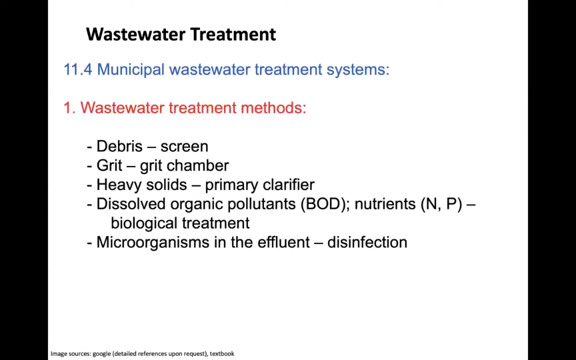 systems first. The first is the wastewater treatment plant. Let me just summarize this one, which was here Just to summarize what this video has said. So here I'm listing the components that were mentioned in the introduction. So, for example, if we want to remove very large debris, right, we're going to use the 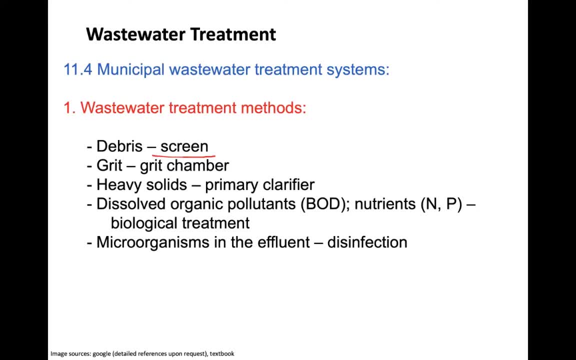 screen, Right. So basically the bar screen, Exactly Right, these larger chunks of contaminants, let's say wood or larger pieces of equipment. so after these larger parts- basically solids- are removed, there are particles or solids that exist in the medium size range, right? so we're going to use a grid chamber to basically remove these relatively. 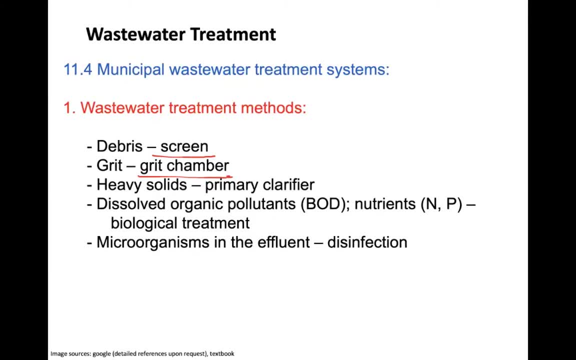 large particles, for example a sand grain, right, so they cannot get blocked by the bar screen. right, so in the grid chamber they can basically settle down or use some inertia to remove them. so then these pre-treated water will go into a primary clarifier. so basically these steps are called the primary treatment. okay, so i'll just write it first: treatment: 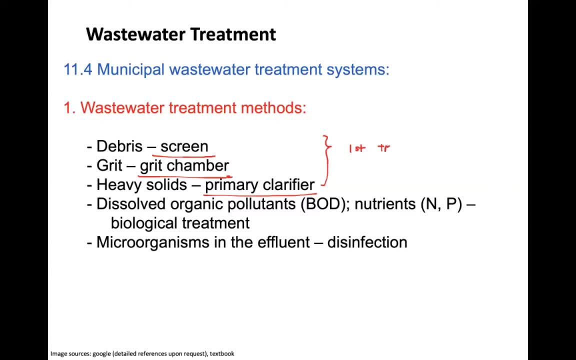 okay, so basically this is categorized as the primary treatment. so for some wastewater, if they have very good water quality, we can just go over the primary treatment, then discharge it back into the nature. but the federal requirement is that for the municipal wastewater we have to go through the secondary or even the tertiary treatment. right, so the secondary treatment? what? 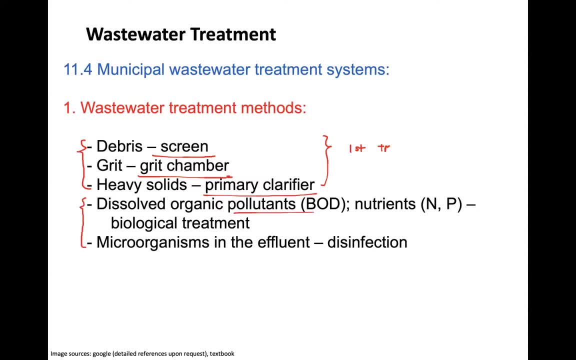 it does is it's going to remove the organics. so if you consider here, here we're just using the physical methods, right, so it's either blocking them or letting them to settle down. but in terms of the chemicals, we didn't deal with the bod at all. 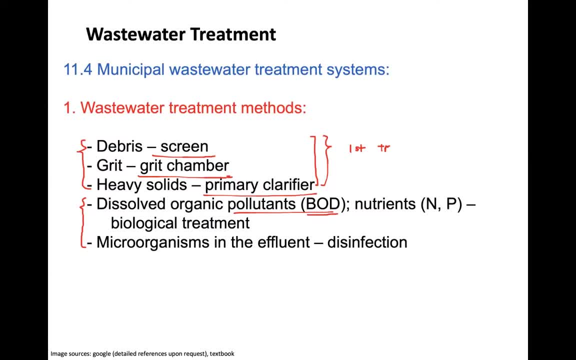 right. so because of that we have to use the aerated chamber or the biological treatment, so basically to send in these uh aerobic or bacteria to let it do the aerobic reaction right, to introduce oxygen and also provide, since we have a lot of organics inside so the bacteria can just consume the oxygen and also consume the. 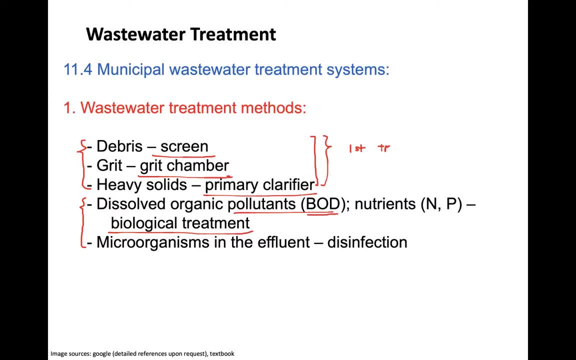 organics so that they can basically reduce the BOD or the concentration of the organics. So in that way we can remove the carbonaceous species and also the nitrogen, the phosphorus species, right? So this is basically categorized as the secondary treatment And then for the 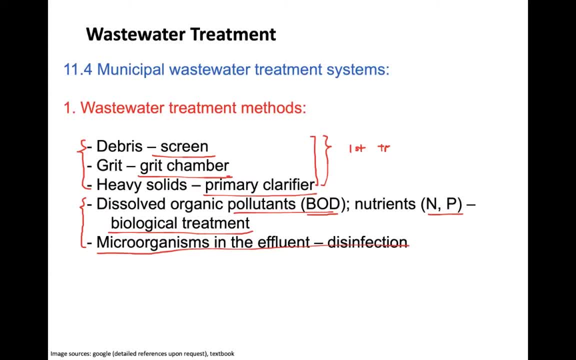 tertiary treatment we can have the disinfection. So basically to further remove the pathogens, to remove the bacteria. Actually, we introduce bacteria in the second method, in the second stage, right, So we have to get rid of them before we discharge them into the nature. So that's why. 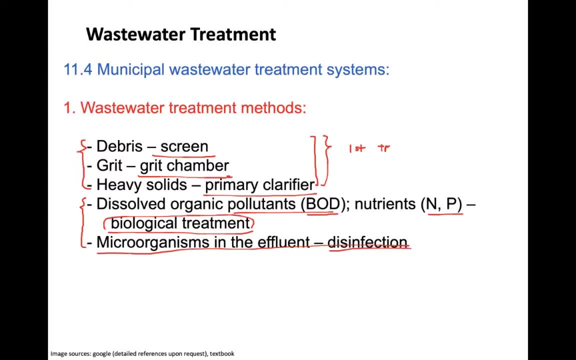 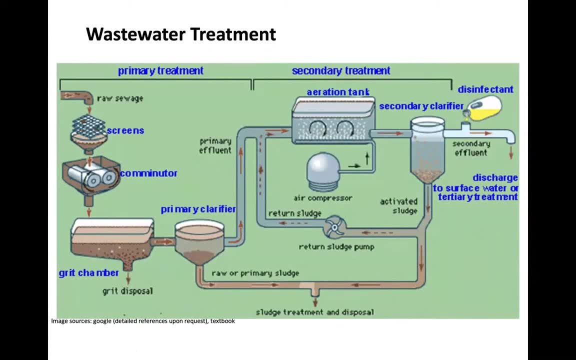 we need to use the disinfection to basically kill these pathogens or these bacteria. So here I also have a schematic diagram that's showing this wastewater treatment process. So basically it starts with the raw sewage. right You can use the bar screen- typical screens- to remove the larger solids And then for some of the wastewater treatment. 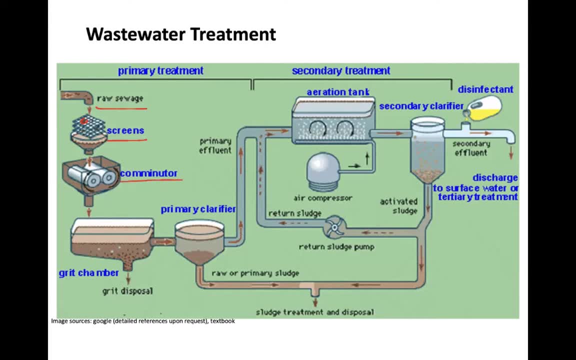 plant. they also use the culminator. So what the culminator does is it basically breaks down the relatively large chunks of solids into grids, into smaller or medium-sized solids. okay, So there are blades. that's attached onto these columns here And then. 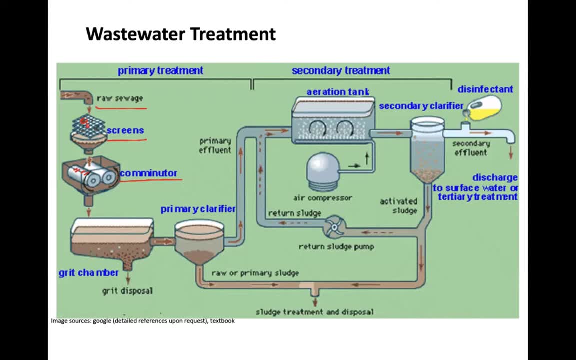 while they rotate they're also attached onto these columns here, And then, while they rotate, they can cut these larger particles that penetrate through the screens into particles with medium sizes, And then basically it's composed of the sewage but with medium-sized particles, And then 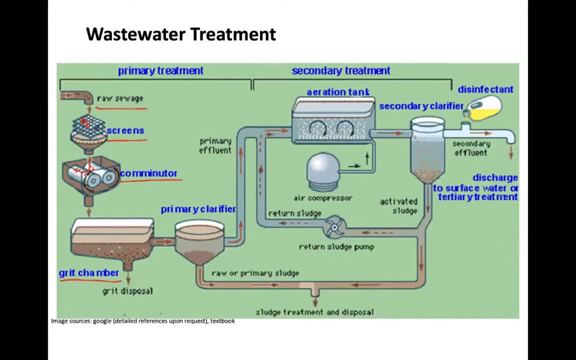 it's introduced into the grid chamber to further remove these medium-sized particles, okay, And then the treated water will go to a primary clarifier. So, as it introduced in the video, what the clarifier does is it's just going to allow particles to settle down based on gravity- okay, So it's very similar to the 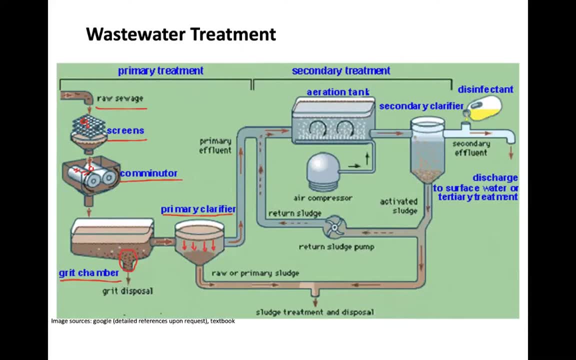 sedimentation basin. that we learned in the water treatment facility right. So when we do the coagulation, flocculation, and then we introduce the treated water into a sedimentation basin, So that's allowing the particles to settle down based on their gravity. So it's very similar in 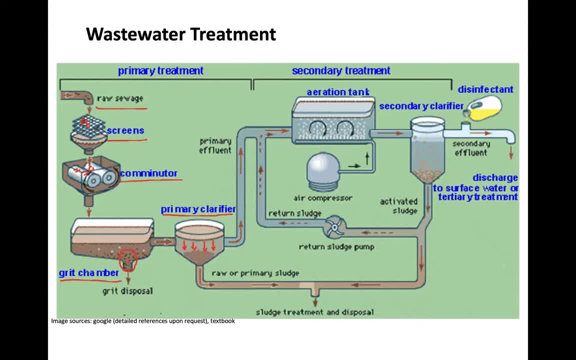 this primary clarifier. It's just allowing the smaller particles to settle down onto the bottom, So this is called as the primary treatment. The primary treatment does the bar screening, does the cutting of the particles, does the grid chamber process and the primary clarifier. 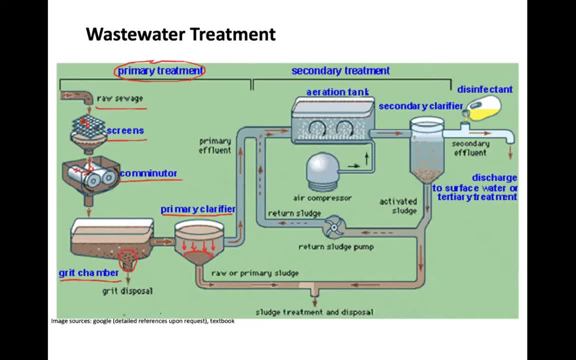 And then, if we worry about the chemical species, let's say the BOD, or nitrogen or phosphorus, what we're going to do is we introduce them into an aeration tank. okay, So this is going to go through the biological process. 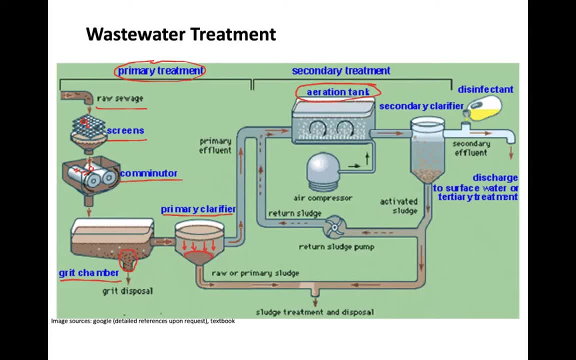 But before we introduce water in there, we know that because of the high BOD, there shouldn't be any bacteria inside, And because of that, what we're going to do is we can introduce some bacteria into the pipe here, okay. So, for example, they can be E coli or they. 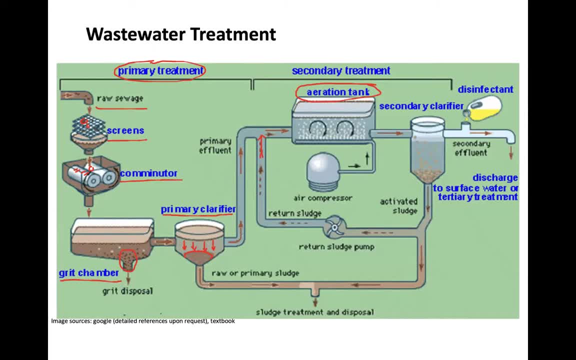 can be some other benign microorganisms which can consume these organics, let's say consume the BOD Right. So this is the introduction of the bacteria. And inside the aeration tank what we do is we have an air compressor to continuously bubble the air, bubble oxygen into the tank. So, as I said, 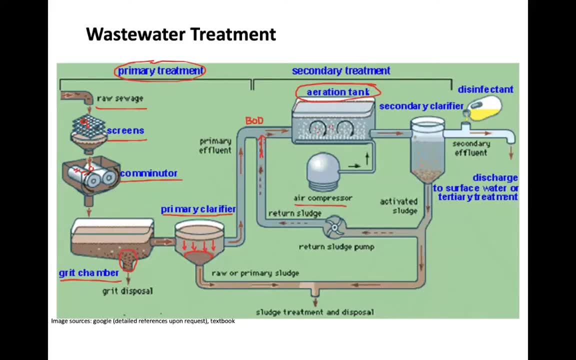 in the video. you can think of this process as the, let's say, the happy bacteria that can have unlimited amount of food, right, Because we have a high concentration of the organics. So we have the bacteria. even if they're in small amounts, they can. 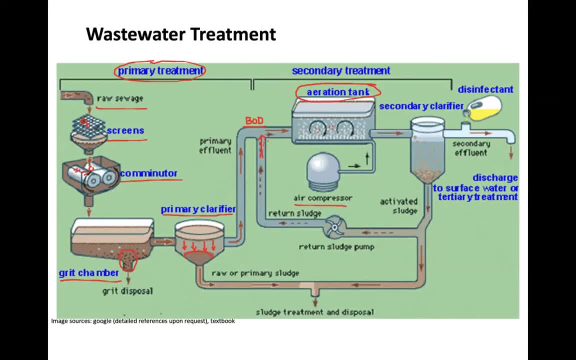 quickly populate themselves right to increase their number into a very large population, And then we can efficiently reduce the concentration of the organics And after, basically after, the BOD is reduced right, so they are guided out and then they're. 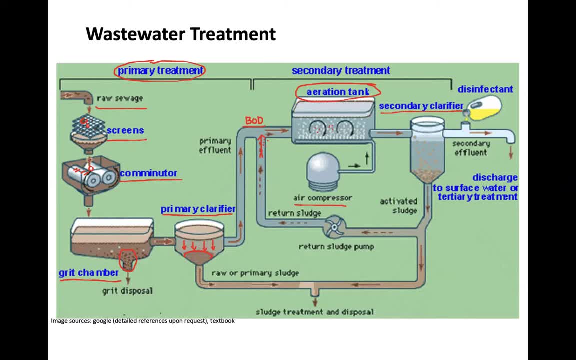 sent to a secondary clarifier. So if you recall the primary clarifier, basically the clarifier removes particles based on gravity, right. And because we're raising a lot of bacteria in the aeration tank, they are going to grow in their size, right, They can form chunks of bacteria. 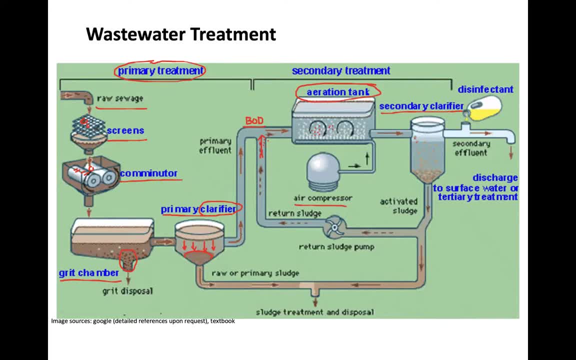 So basically in the secondary clarifier these larger chunks of bacteria. they can settle down and then form these solids And then at the top is going to be relatively cleaner water And then we can send them through the disinfection right. We can add in the, let's say, either chlorine or 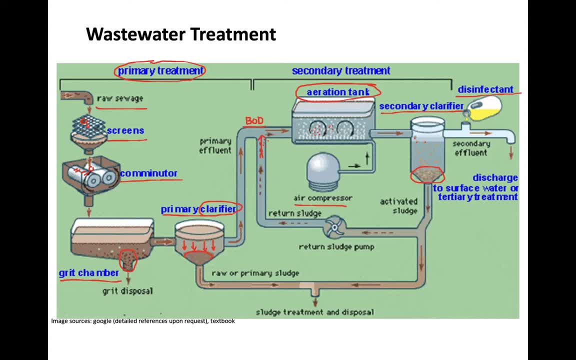 we can add in ozone or or UV disinfection to further purify the water. But, as you can see, the secondary treatment is mainly dealing with the aeration tank and the secondary clarifier. okay, So the disinfection is categorized as the tertiary treatment. So, basically, the water coming out, you can further 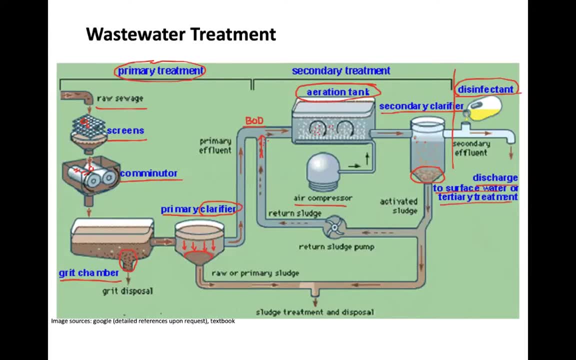 basically, you can just discharge them into surface water or you can go through more tertiary, tertiary treatment processes. So now we deal with the water right, So we basically come up with relatively cleaner water from the raw sewage. This is clean water, raw sewage, okay. So what happens to the solids? Okay. so how are we going? 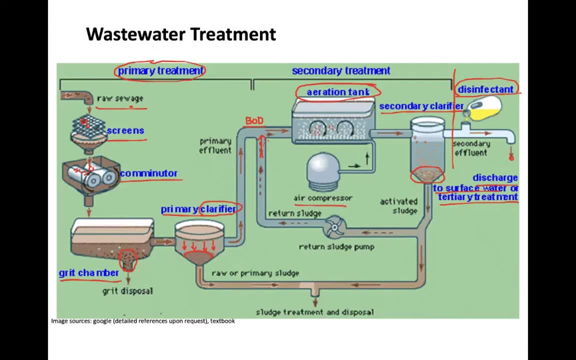 to deal with the solids that are coming out. So the solids are, some of them are in the in the sparse grids, So we can directly dispose them in the landfill right. But in terms of the solids that's coming out of the grid chamber, they actually form. 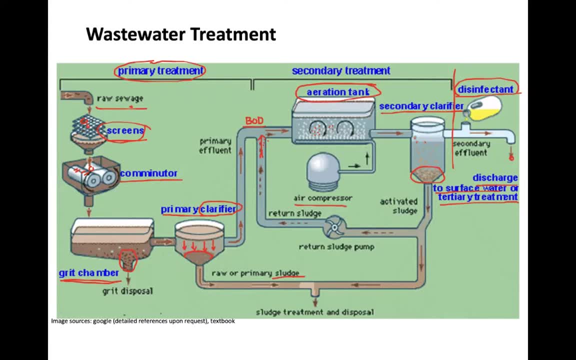 something called the sludge. So basically we have the solids, but also in the solid there are some water inside, But so before we dispose them, we have to first dry them right. So this is what comes out from the primary clarifier And in terms of the secondary, 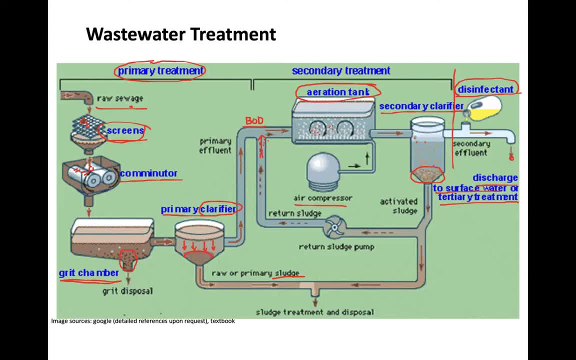 clarifier, if you consider what is the major composition here. so of course there may be some, let's say, suspended solids that are basically not removed by the primary clarifier, But more importantly, there are a lot of bacteria inside right, Because we basically culture them. 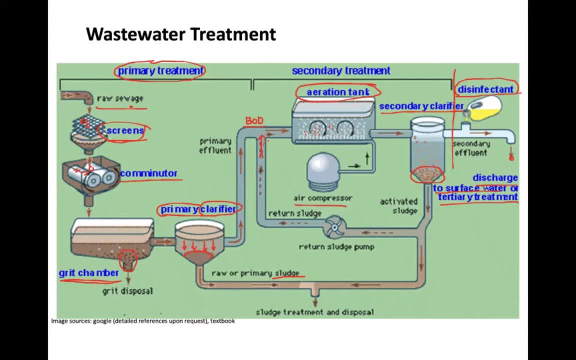 in this aeration tank here. So their population grew a lot to form these larger solids. But if you imagine, at the beginning we have to introduce some bacteria into the aeration tank, right. So what that means is we can split a fraction of this solid, So what people call activated sludge. okay, 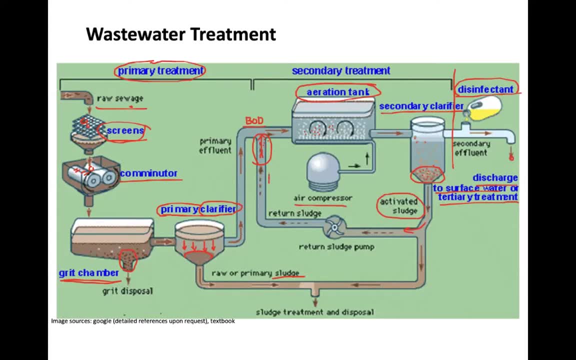 fraction of it and then send it back into the inlet of the aeration tank, right? so basically, we have a lot of bacteria at the bottom of the secondary clarifier. we can split a fraction of it, send it back into the aeration tank so to enjoy the unlimited organics or unlimited food again. 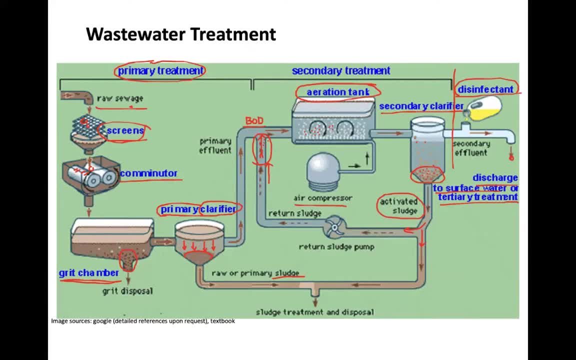 but most of them actually get this disposed okay. so they're going to mix with the primary sludge and then go to the sludge treatment or disposal right. so this is the general process for the water treatment, for the wastewater treatment, and what we're going to do in the following. 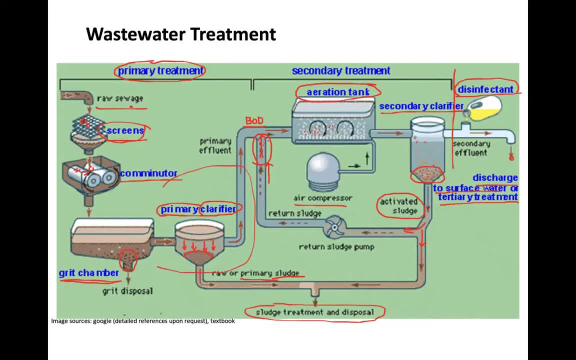 classes. classes is that we're going to do some calculation regarding the primary clarifier and also the calculation regarding the aeration tank, because these processes needs a very accurate engineering because, just think about it, if we send in two high of a flow rate into the primary clarifier, while the flow rate is too large that we don't 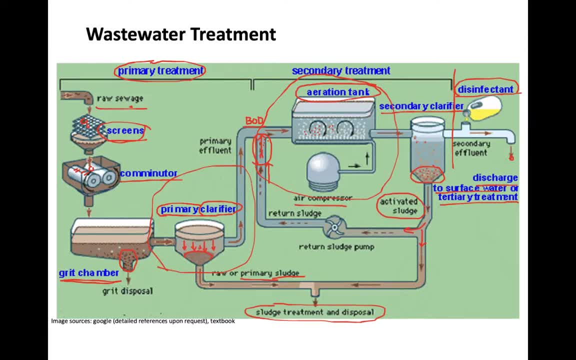 have enough time for particles to settle down, then the primary clarifier is not effective to remove the larger particles. and in terms of the aeration tank, what happens is if we send in too little of the bacteria, then they may not populate themselves enough for the in the aeration tank. and if we pump 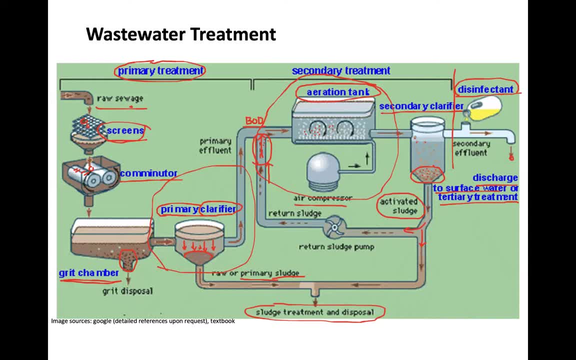 in too much of the bacteria, then at the beginning they don't have enough of the food right, so they're going to get killed and that's also a waste of the waste of money in terms of sending them into the aeration tank. so there needs a lot of engineering calculations here. all right, so this is a general.